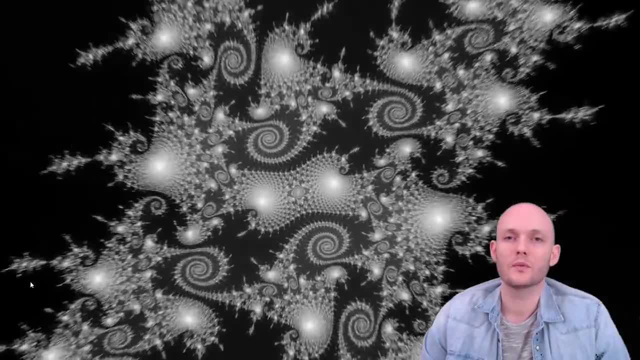 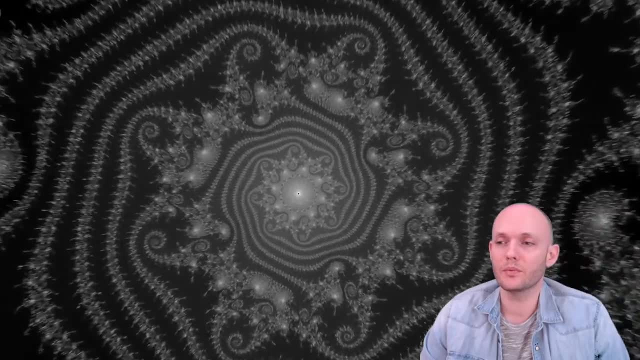 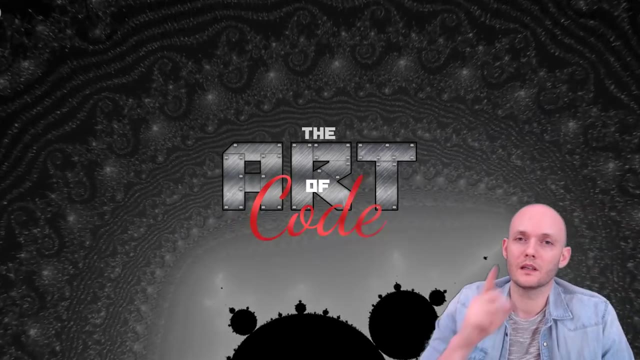 such beautiful images. It is also the go-to example for what you can do with complex numbers, and it's literally infinitely deep, infinitely complex and, in my mind, infinitely beautiful. But how does it work? Let's find out. All right, Wikipedia to the rescue. So there we go. 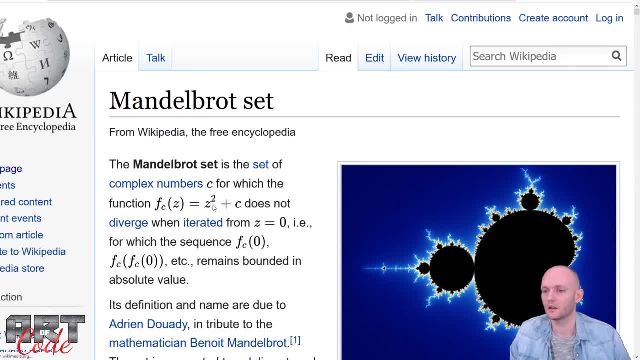 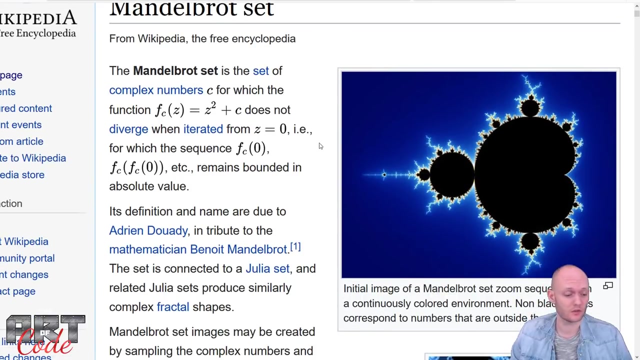 Mandelbrot set- Enter. All right, the Mandelbrot set is the set of complex numbers c, for which the function fz equals z squared Square plus c does not diverge when. Okay, well, there's a beautiful image. So there's that, And maybe we should try something else. 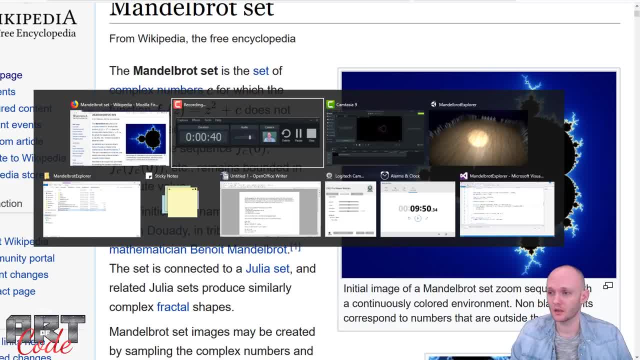 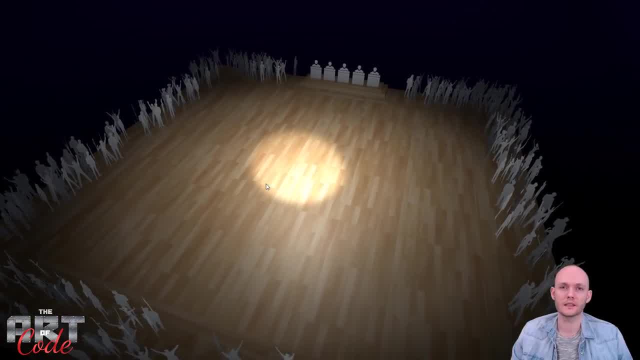 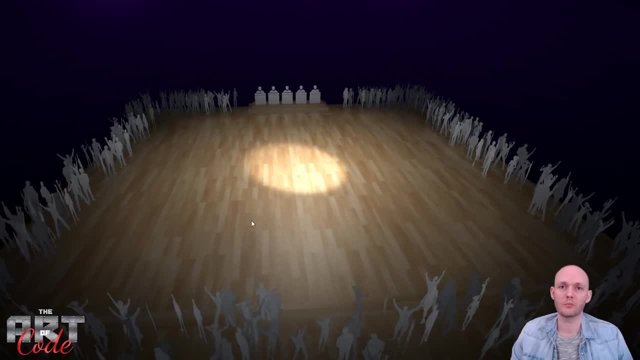 first. So let's do something else. Let's go over here and let's imagine for a moment that we're at a dance competition, right? So here we have the dance floor and there we have our judges. They're going to judge the different couples that are going to dance, And I have the option here to 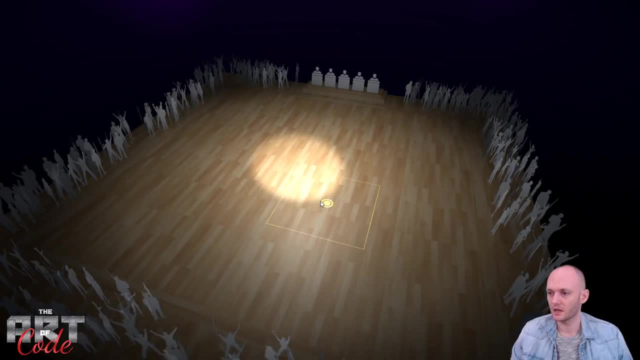 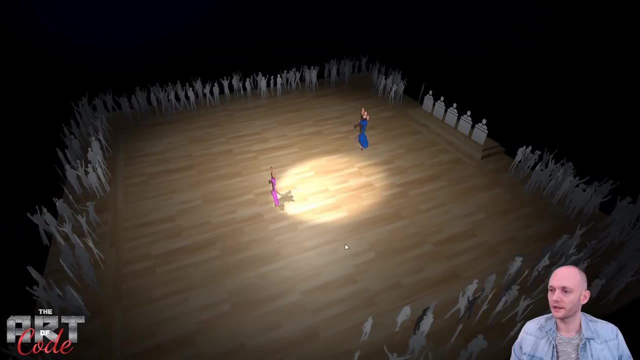 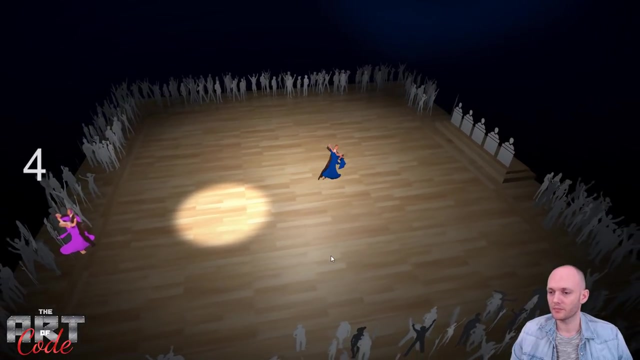 put couples in different spots on the dance floor. So I can, for instance, put a couple over here and I can put a couple over here and I can let these couples dance and see how they do. And these couples are going to get judged on how many steps they do before they screw up and go outside of the. 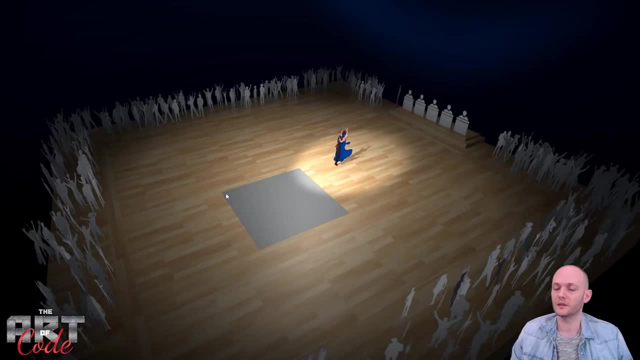 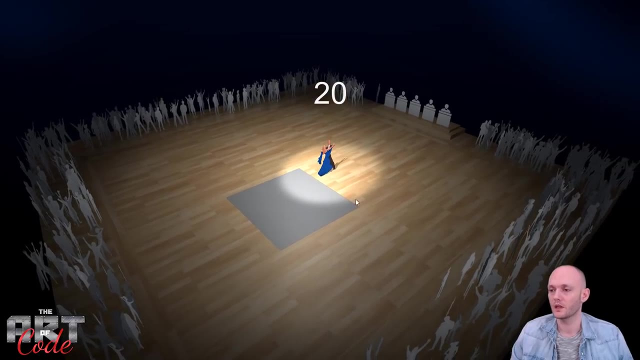 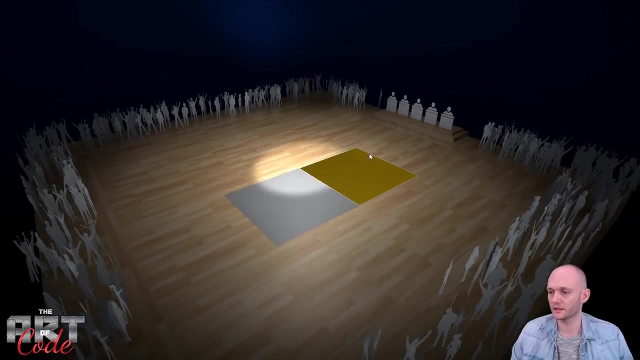 dance floor And when they do that like that, the part of the dance floor where they started gets graded or gets colored based on the number of steps that they took. So these guys, they never went outside of the dance floor, They went to the maximum number of steps allowed in this dance competition. Otherwise it would take an 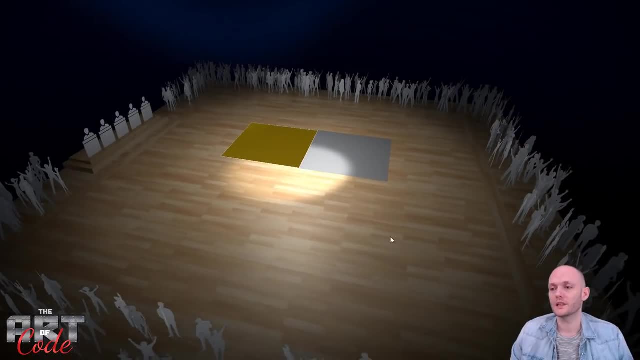 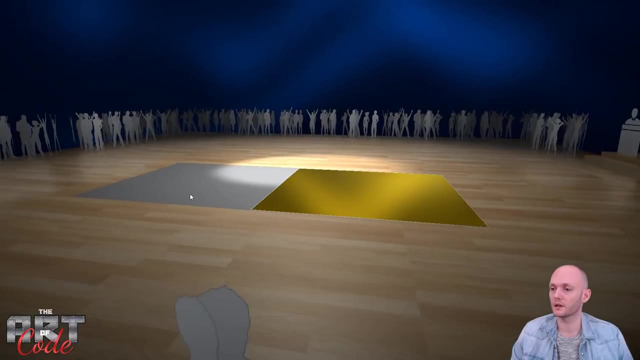 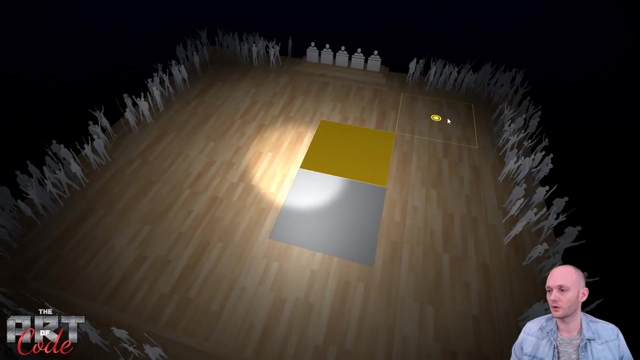 eternity, literally. So they went to 20 steps. So therefore they get a gold medal and we make the part of the dance floor over there gold. so let's put some more couples here and let's see what this entire dance floor looks like. 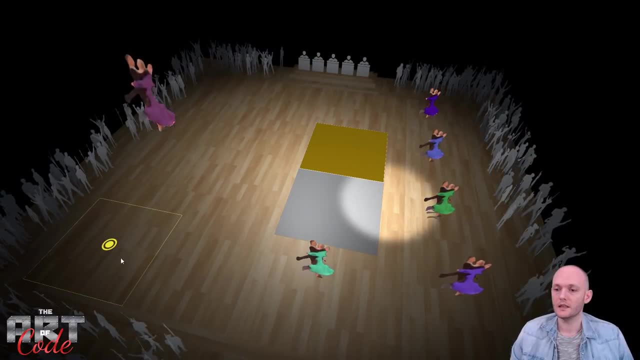 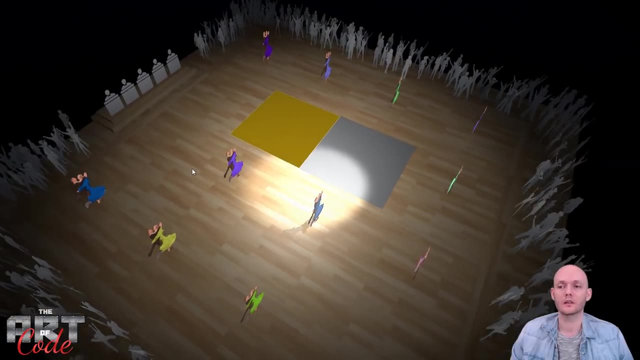 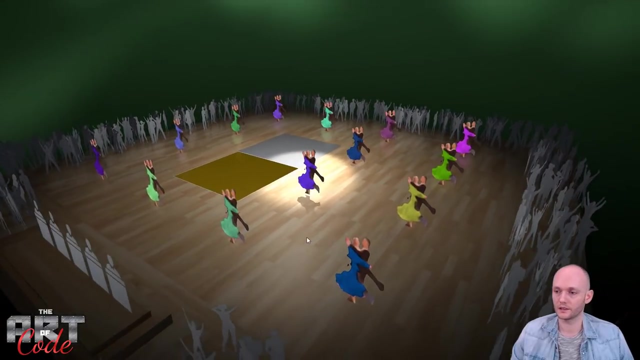 and as i'm putting these couples, i must say that the the dance steps that these couples are are doing are are mathematical dance steps and they're all the same, and the only thing that that is different is that these couples start in a different position. they start their dancing. 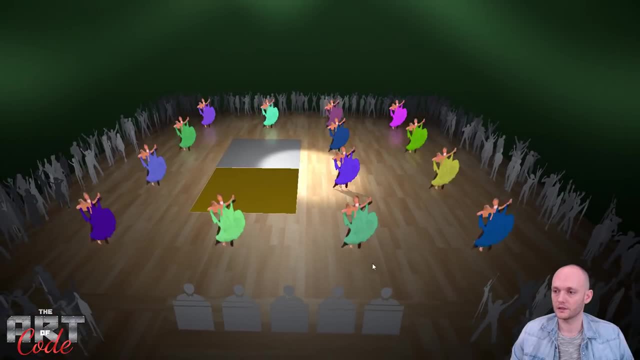 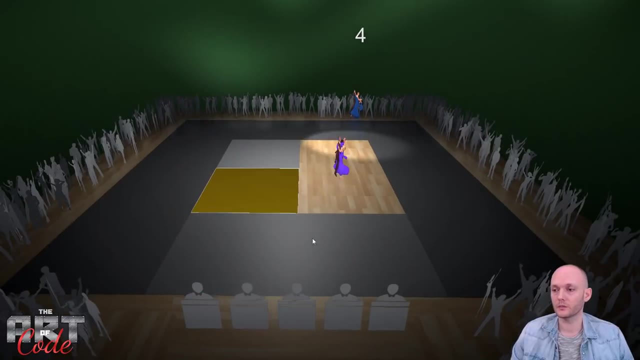 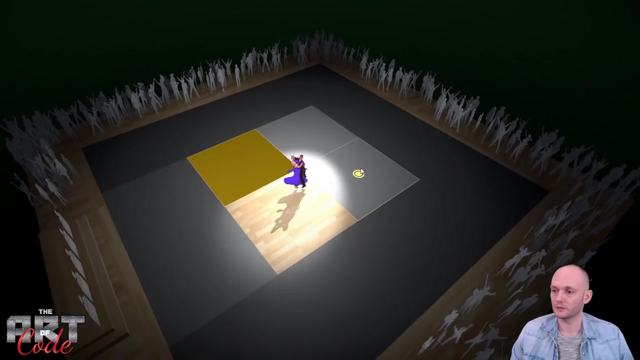 in a different position. so all right, here we go. let's see how these guys do so. most couples screw up right away, but there's there are a few that go a little bit longer. so up here were were two that went a little bit longer, over here there was one that went a little bit longer, and over here there. 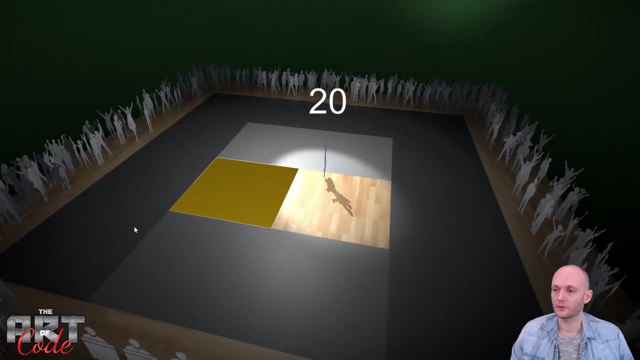 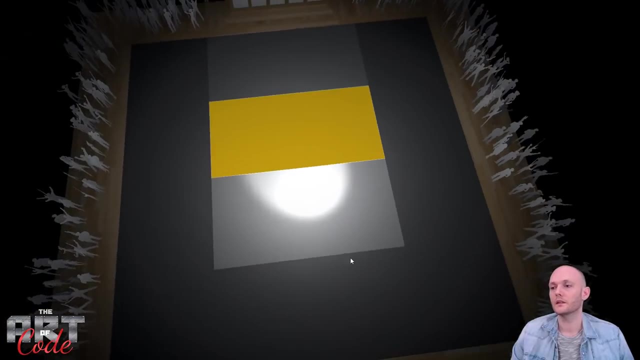 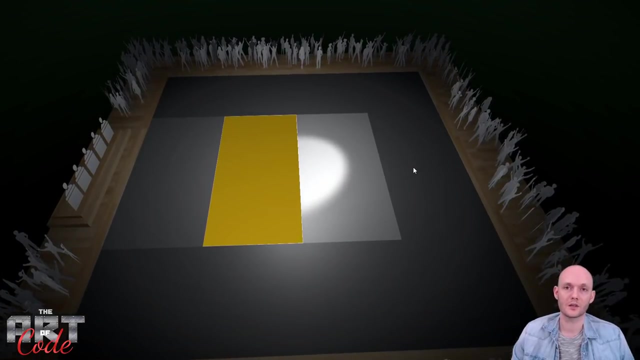 is one that will probably go the entire 20 steps. so there we go. so that's also going to be gold, and you'll see you that a certain pattern is starting to emerge here, and i said before that the only thing different between these couples is where they start their dance, right. so, and right now, the dance will start. 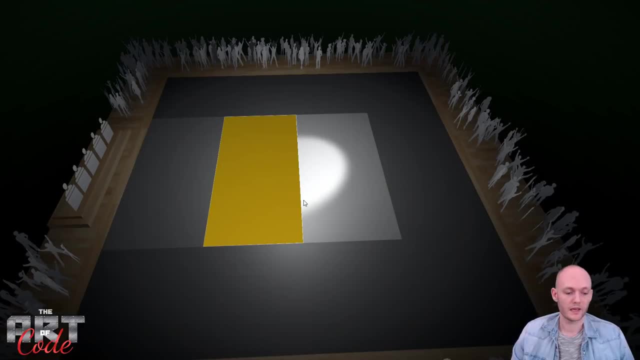 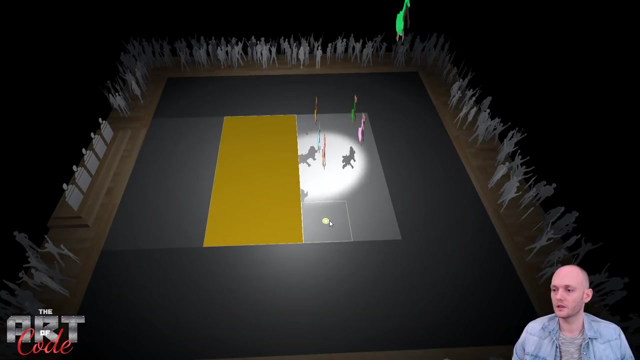 at in the middle where the yellow circle is. but i can make this area smaller. so if i make this area smaller, so now i can put four couples where before there was only one. so let's put four couples. so one, two, three, four and actually let's just put eight. 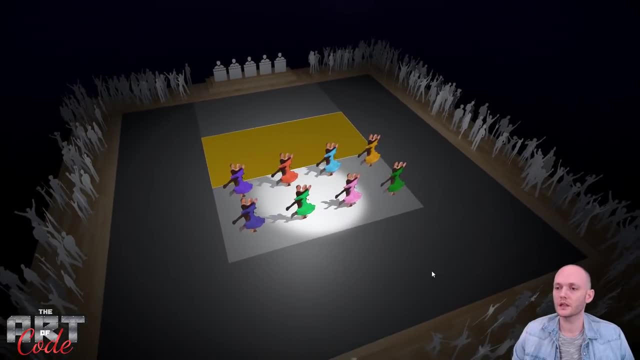 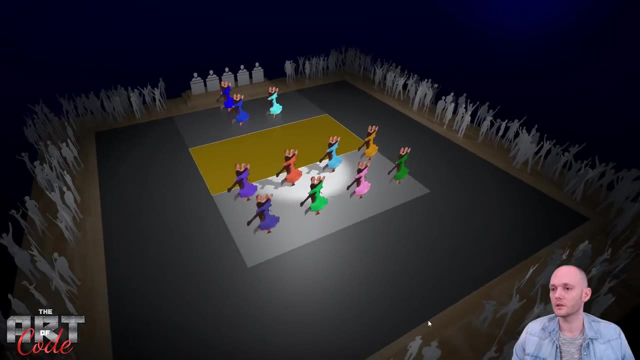 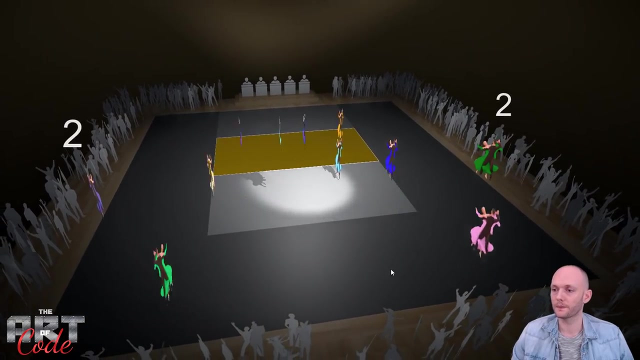 and see what that does. and actually, while we're at it, let's just put a few more over here as well. all right, so now we have- oh, i missed one, let me go over here- so now we have a total of 12 couples, so let's see what they do. and they start dancing and a lot of them kind of screw up quite quickly. 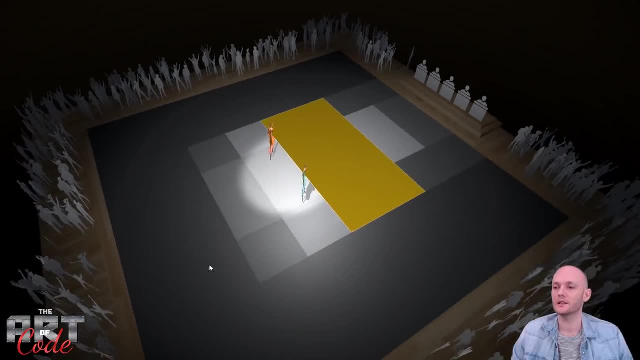 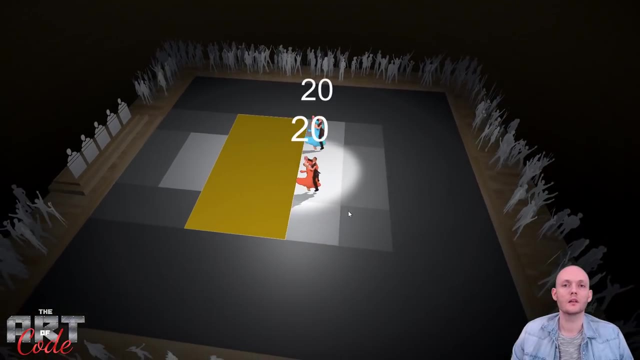 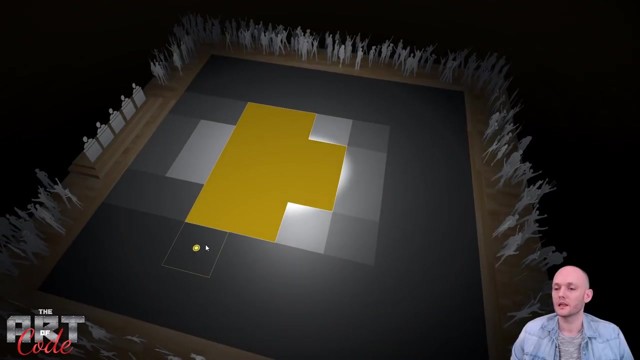 but we'll see that this pattern is starting to refine itself and these guys will probably go all the way. and now i can put smaller and smaller, or i could put dancers on smaller and smaller areas, but if i put them one by one, we're going to be here all night. so i made something where i could put a little army of dancers down. so so now 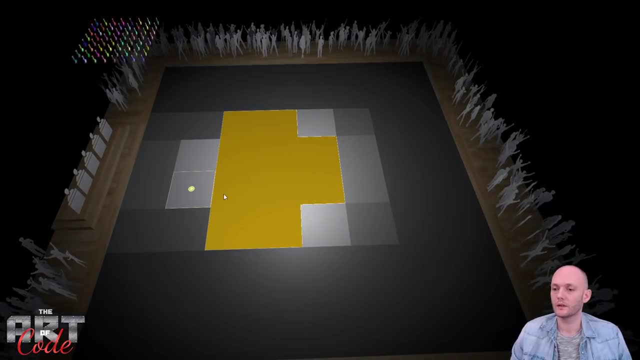 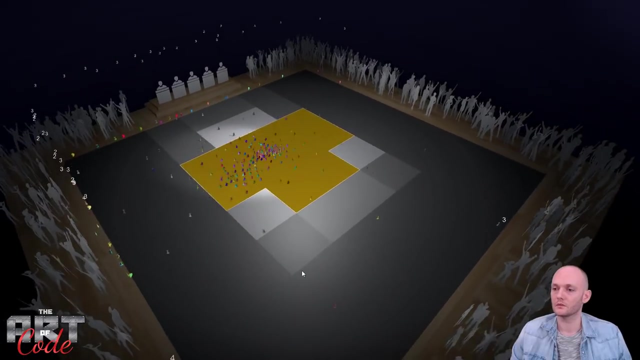 instead of putting only one dancer, i can put 64 dancers at once. okay, so 64, 128. so now we have 256 dancers over here. so let's see what they do, and i hope my computer can handle it, so we'll see. okay, so there's a lot. 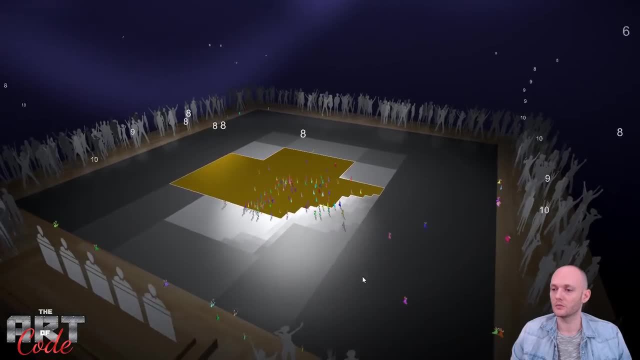 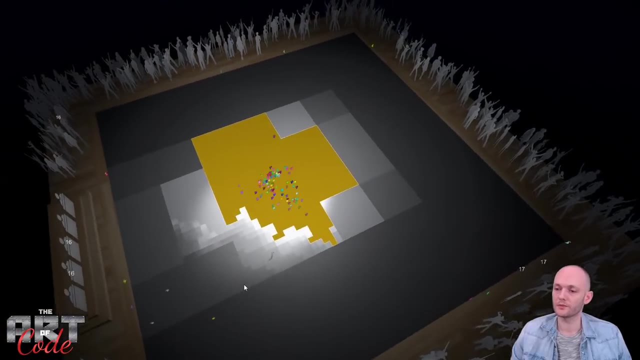 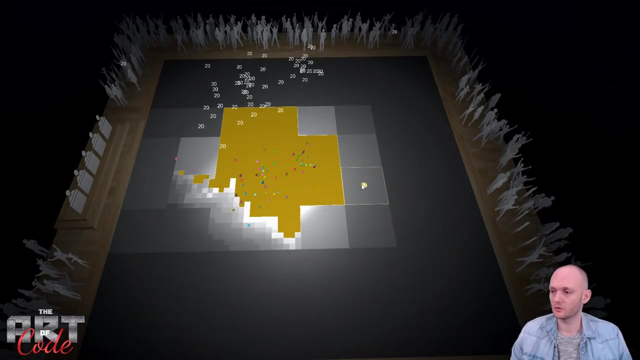 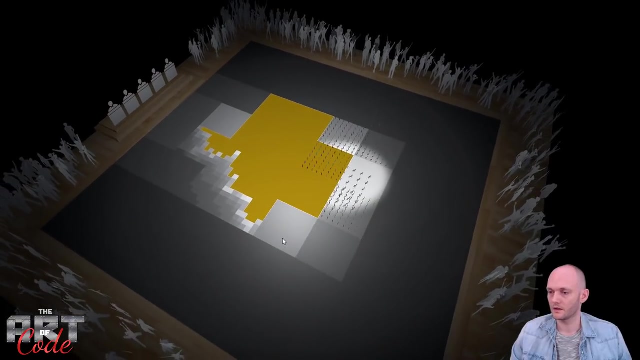 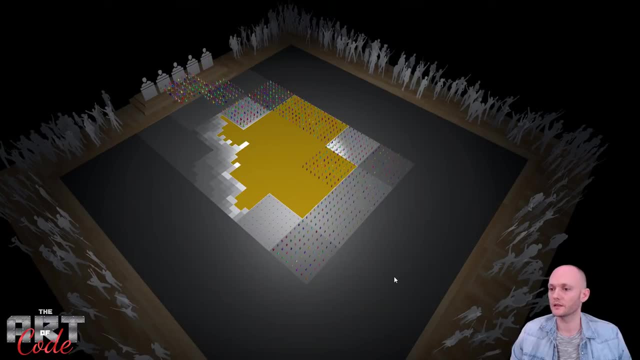 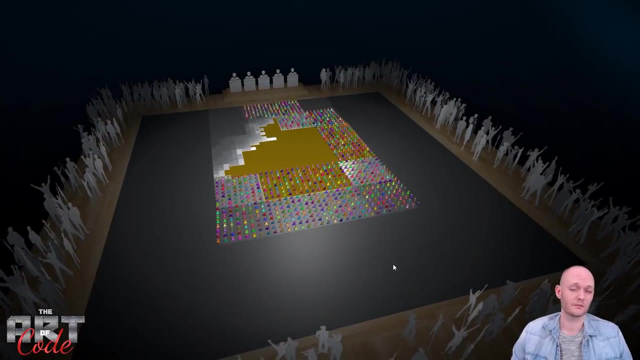 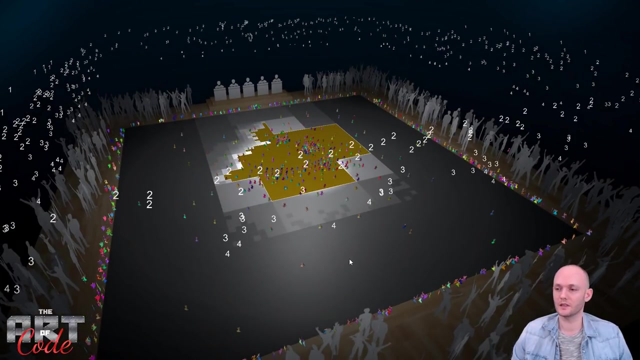 there, my computer is going to explode, but at least we're going to get somewhere with this, and over here as well. all right, so this is the end of my computer. oh well, so far, so good. yeah, now it's starting to chop like crazy. you can do it. 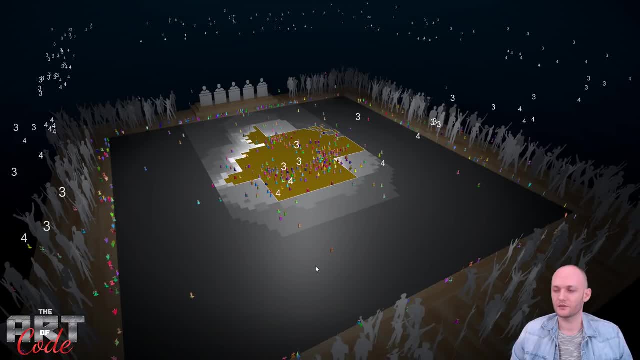 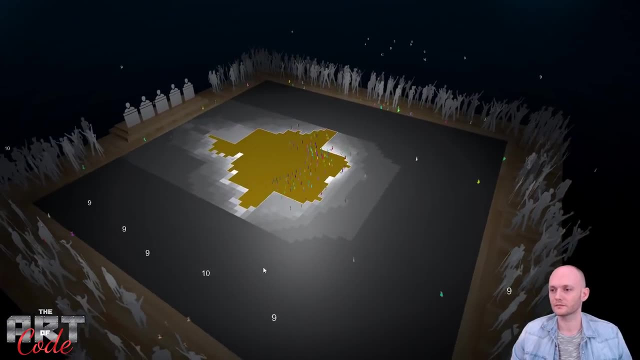 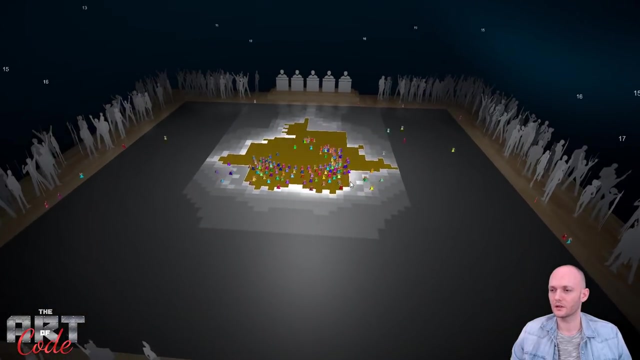 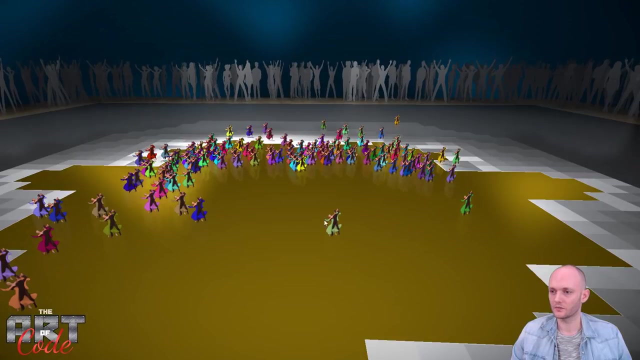 you can do it. crash through it all right. so we're still going. a lot of them are still going. a lot of them are also. they seem to be stationary, and there we go, and now let's get the score for all of these guys. you can do it. 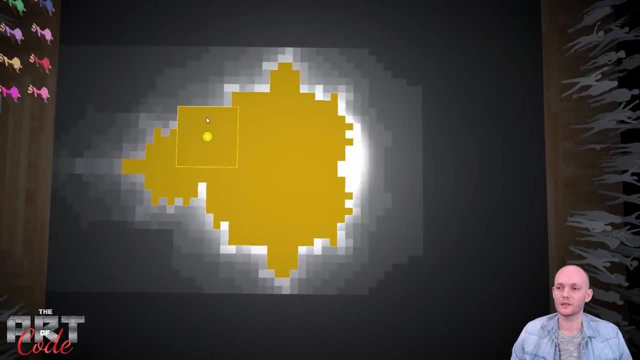 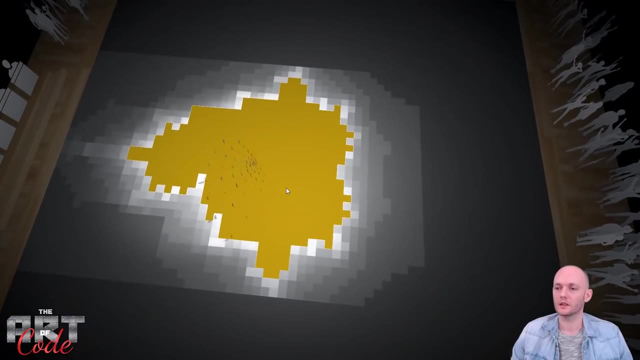 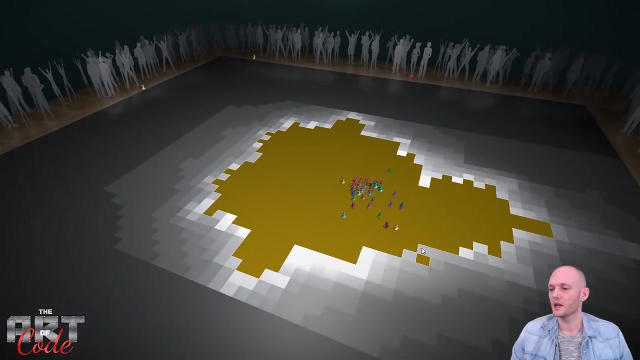 all right, you can see that a certain pattern is starting to emerge here. that is obviously the mandelbrot fractal, so that's kind of how that works, and the cool thing is that, well, i should have maybe wait until these guys are finished, but i can zoom in and i can put. 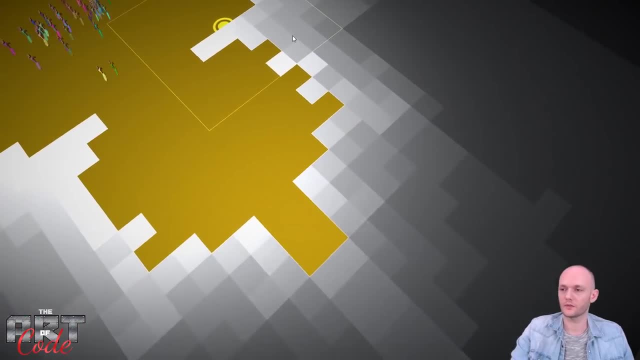 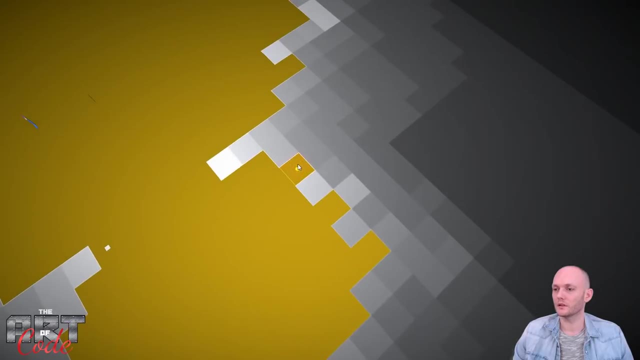 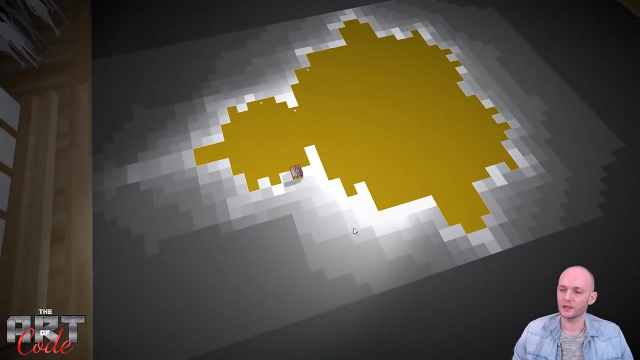 smaller dancers or i can put dancers on a smaller area. so if i go over here and let's say i take, i take a point over here and I put 64 dancers on that tiny little spot over there, you will see that they start out dancing very like synchronized, as as one unit almost, but very quickly, after very few steps. 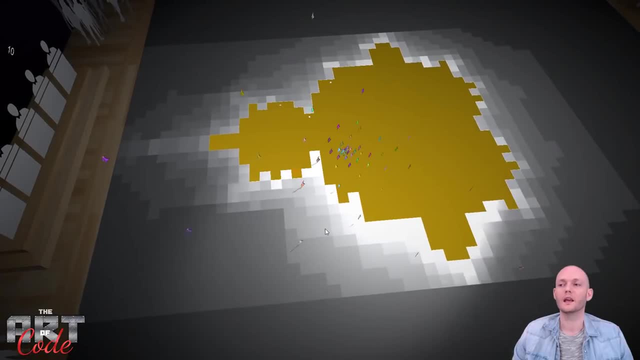 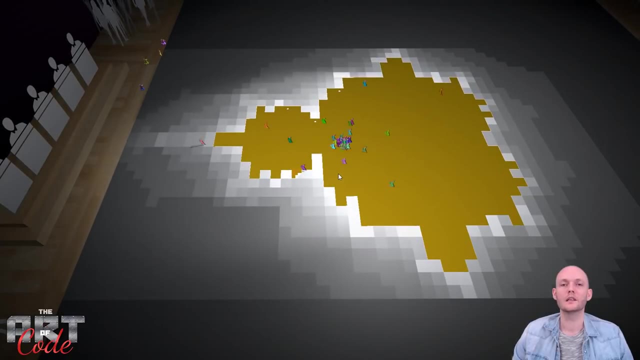 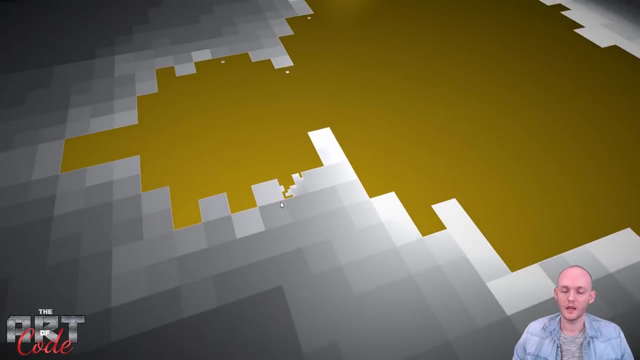 their behavior will become very erratic and all of them will go in different directions. and this is kind of the idea behind chaos is that really small differences in input will will result in really large differences in output, and so that just made this little tentacle over here, and if I would keep 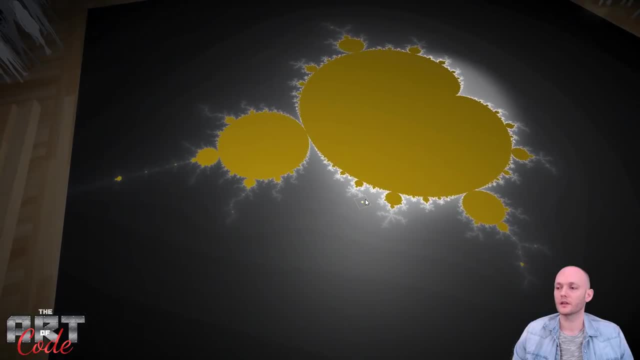 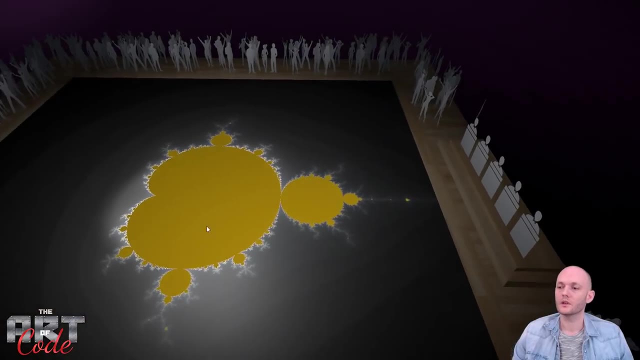 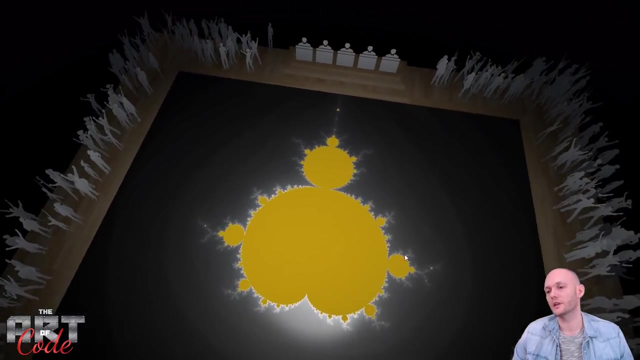 going, then we, in the end, we would get something like this: isn't that beautiful, alright. so this making- I'm making up this image- has a few different ingredients, right? so like the first ingredient would would be, for instance, which part of the dance floor we're visualizing, right, right? 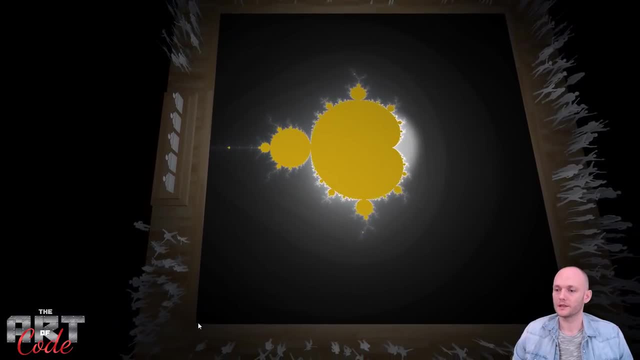 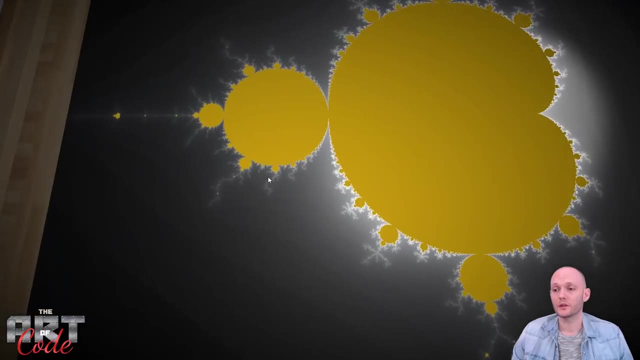 now we're visualizing an area that goes from minus 2 minus 2, 2, 2, 2. that's a nice sentence, but we could also, obviously, visualize a smaller part and just let's say, get one, one of these spirals, or what have you right? 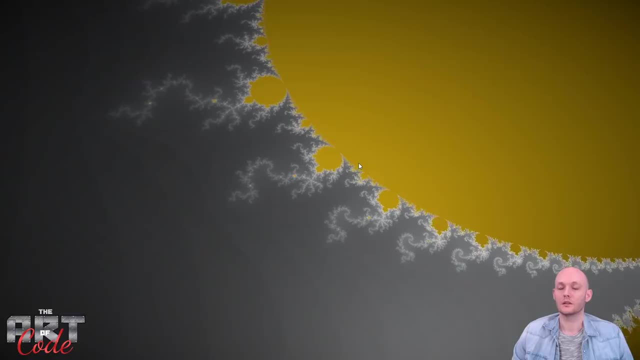 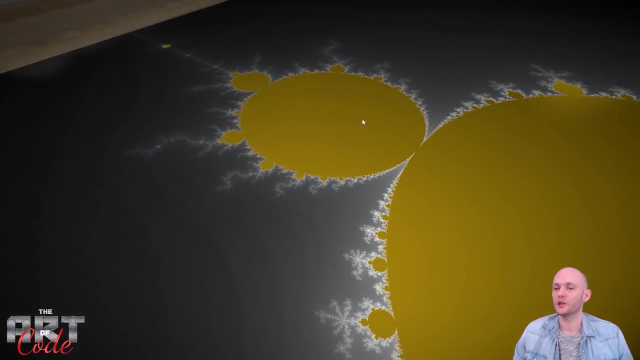 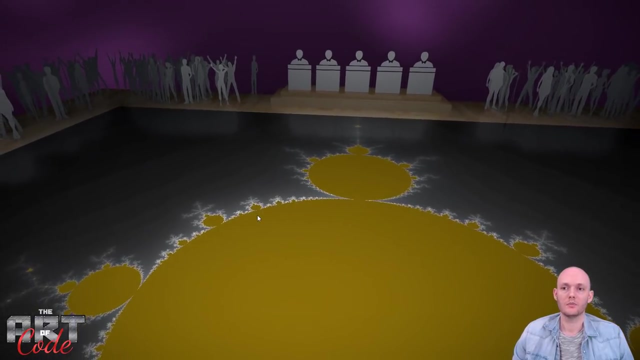 we can rotate and do all kinds of stuff. so so that's one ingredient, which part of the dance floor we're visualizing. then there's obviously the judging rules. right, so right now, the judging rules were well, however many steps it takes before a couple screws up and gets out of the dance floor. 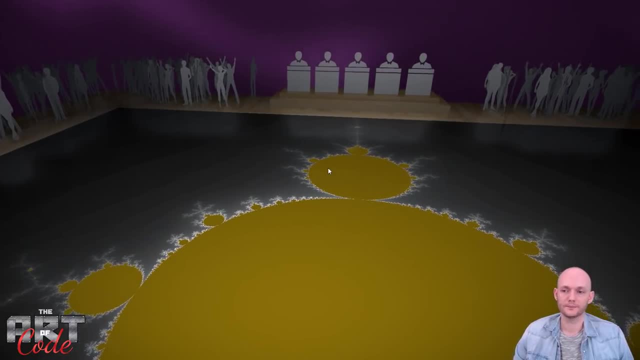 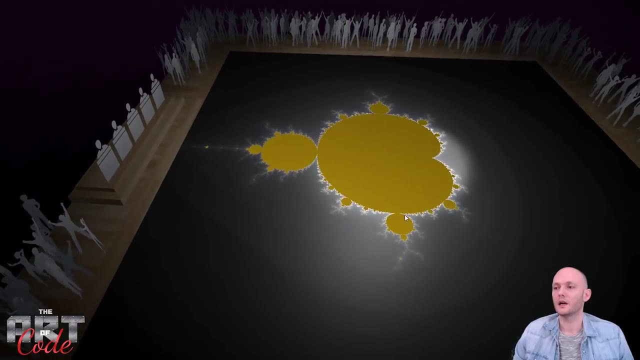 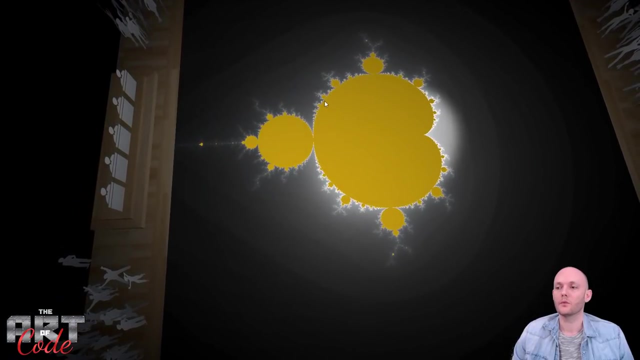 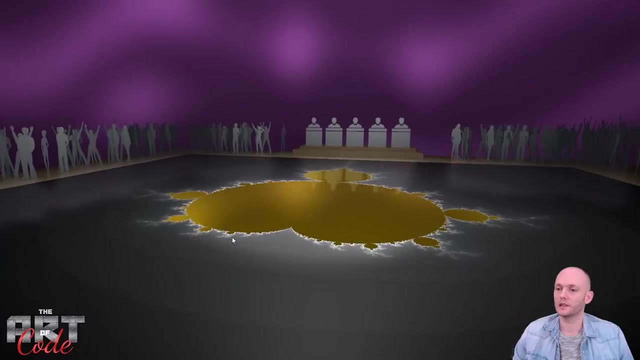 but there could be different rules. we can look at that later. then obviously, there's how the results are visualized, right. so so how do we turn a score into a color? so normally, or what happens very often, is that when it's inside of the amount of outset, they color it black. in this case, I colored it a nice shiny gold and you 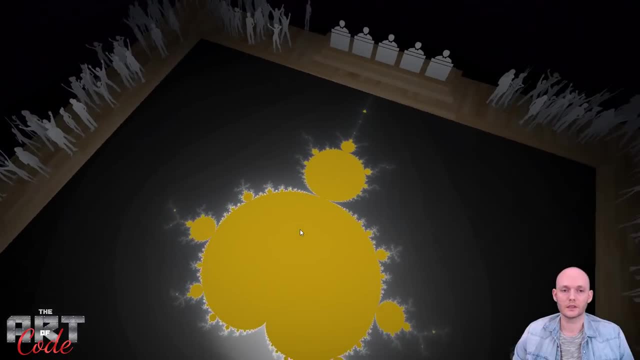 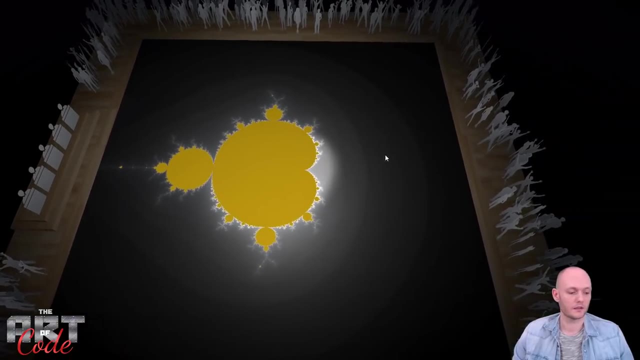 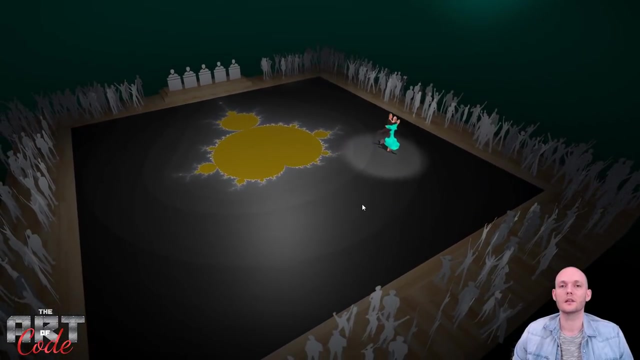 can color at any color of the rainbow, so we can also look at that. and then, last but certainly not least, is that dance step right? so so what rules are useful to make a dance floor? and the question is: do these couples follow when they start dancing? so let's look at that. so, if you just go back to 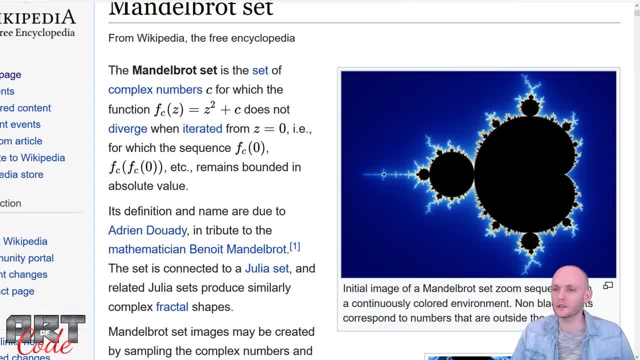 Wikipedia for one second and we read this again. maybe now this makes a bit more sense. so complex monitors, for let's forget about that, but let's say here, look. so basically, it, it, it. it runs this function here, which is the function to get to the next dance step and the Mandelbrot set is. 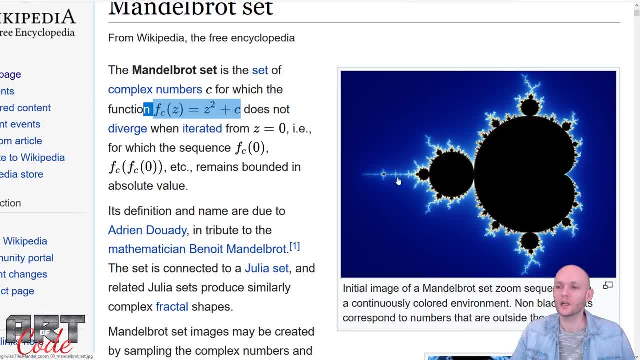 the set of of starting points for which the output remains bounded, meaning for which the outfit doesn't like, for which the dancer does never get outside of a certain limit. so I hope that makes a bit more sense now. so let's take this, this formula here, and let's expand on that a little bit. so we 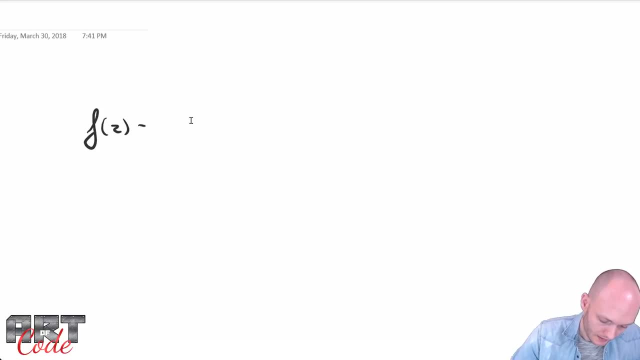 have a meaning. that means come out of the step three. filter of自由. here let's expand to a function down at route 15. now, if we come to the other input, all right. so here you go. there's a. have the f, z equals z squared plus C, right, and let's just point some arrows. 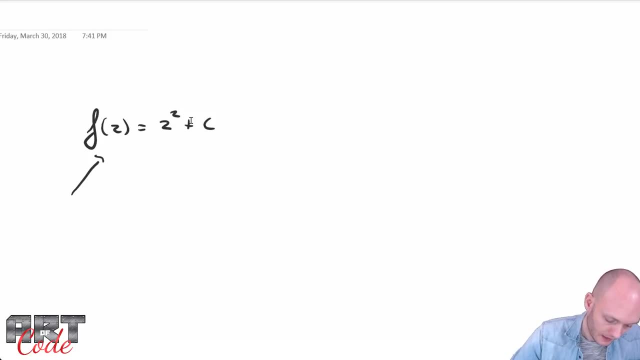 here and say what we're looking at here. so this fz is the new position, so it's the position of the new, of the next step in the dance. then over here we have the current position, all right, and last but not least, over here we have the start. 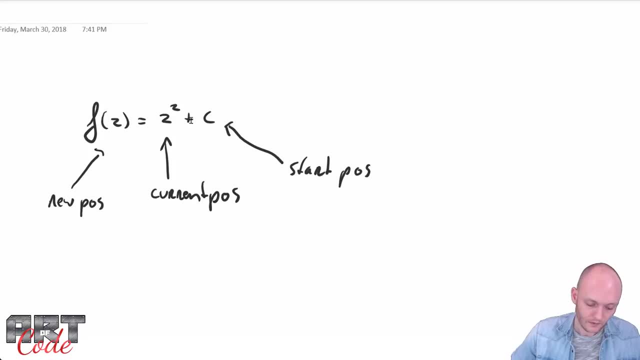 position: all right. and and Z and C are complex numbers. now, what does that mean, complex numbers? well, it might mean many different things. I'm not a mathematician, so like there might be other nuances that I'm not getting here, but what I do get from it. 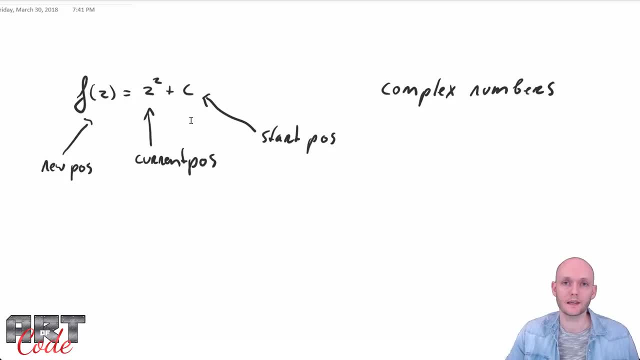 is that a complex number has two parts to it. it's basically like a vector 2. it has an X and a Y component, or, like they like to say, a real component and it has an imaginary component. and I said it's like a vector 2, so the real component is: 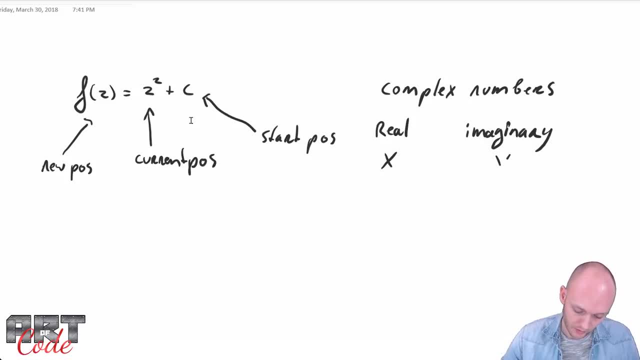 the x and the y component. and the x and the y component are the real components of the vector 2 and the imaginary component is the y component of the vector 2. and this x and y is also the x and y of the image, of the fractal image. 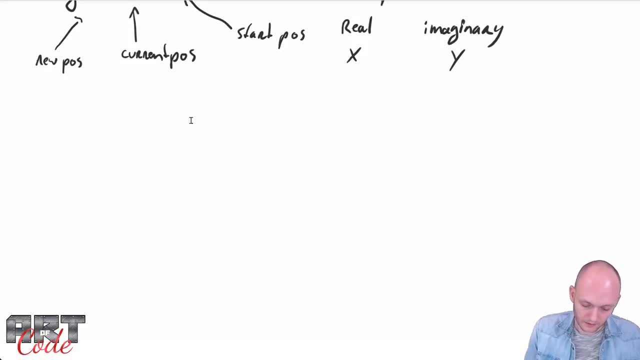 that we're gonna make. so let's just first look at the real component, at the x component. so let's just look at the number line, so this would be the, the x axis, and it has zero in the middle, and then we go one, two, three, four, like 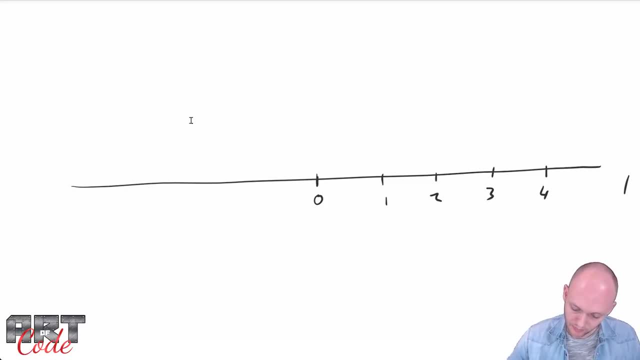 whatever. so one, two, three, four. so this is the positive x direction, and we also have the negative x direction, right, minus one, minus two and minus three, and so on, so forth. this is negative and this axis we'll call this axis the real axis. all right, we also have, in complex numbers, an imaginary component which is 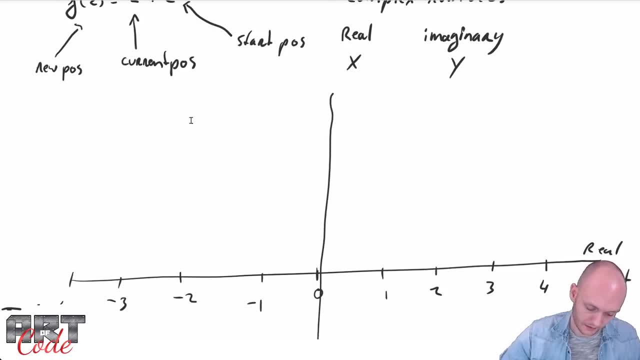 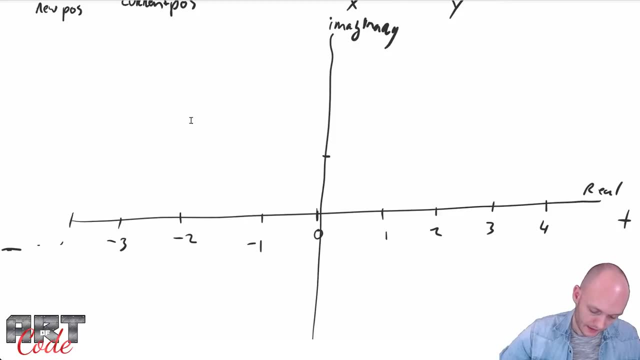 on the imaginary components of X prop喱 axis. all right, so this is the imaginary axis. imaginary and and this also has like numbers going positive over here, and what we like to do over here is say 1i, 2i, 3i and so on, so forth. 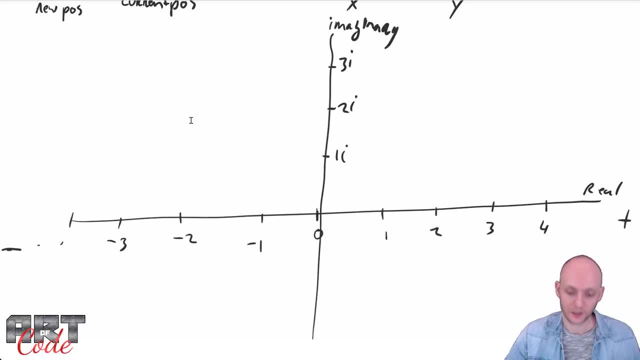 basically that just says it's 1 in the i direction and it's 2 in the i direction. similarly, over here we could say: it's 1 in the r direction, for real right, or it's 2 in the r direction, or it's 3 times. 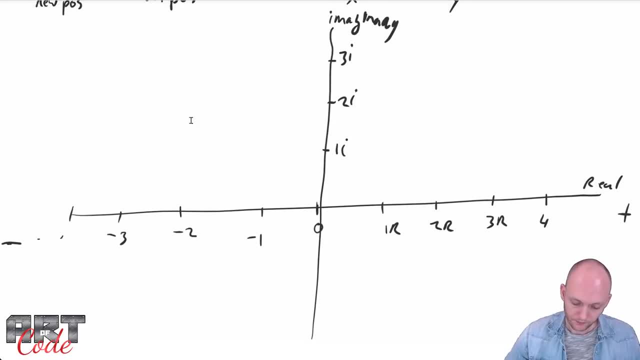 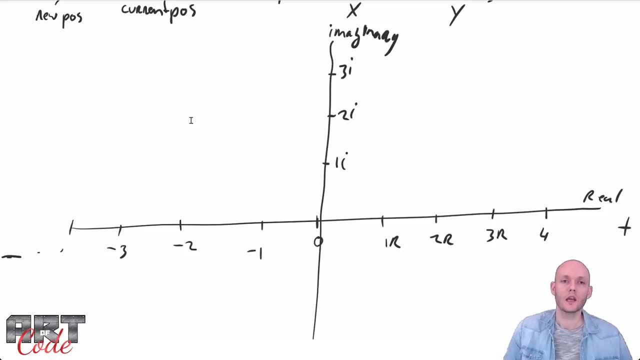 the r direction. and the difference between imaginary numbers and real numbers is that mathematicians have come up with slightly different rules for imaginary numbers than they have for the normal real numbers that we're used to. so for the normal real numbers, you can add them, you can subtract them, you can multiply them and 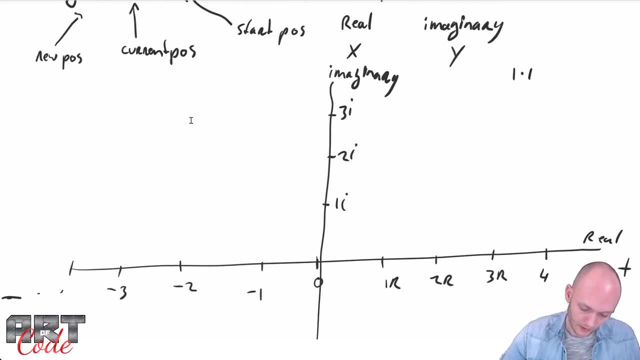 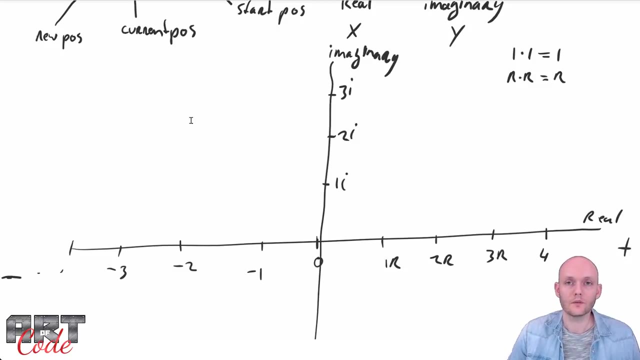 and one of one of the rules is that 1 times 1 equals 1. or we could say, like in this case: r times r equals r. right, 1 times 1 is 1. the difference between real and imaginary numbers is that for imaginary numbers that rule is slightly different. so for imaginary numbers, 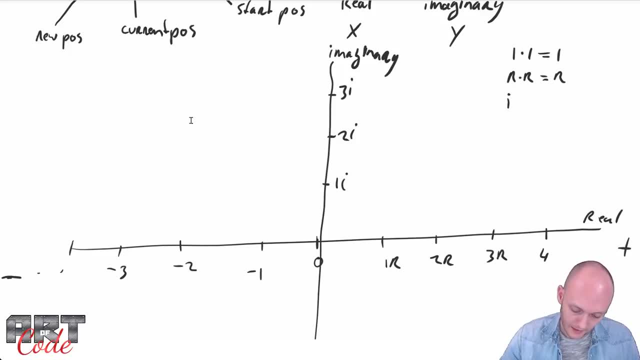 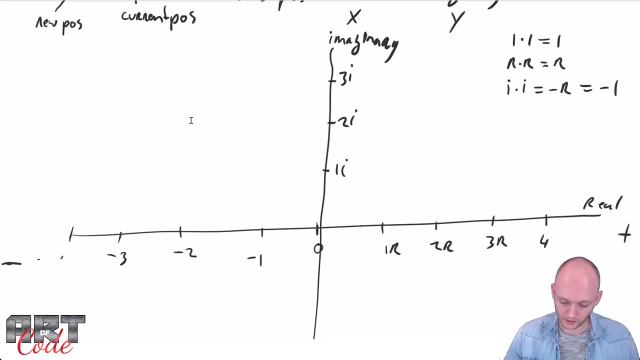 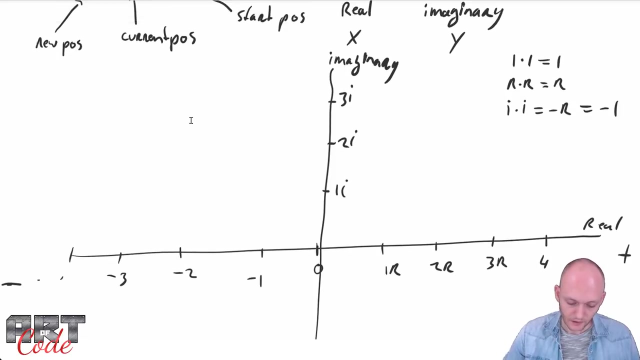 we don't have i times i equals i. we have i times i equals minus r or minus 1, all right, so so let's see. that's as far as i know, that's the only difference between imaginary and real numbers. so let's see how that plays out, because over here, over here. 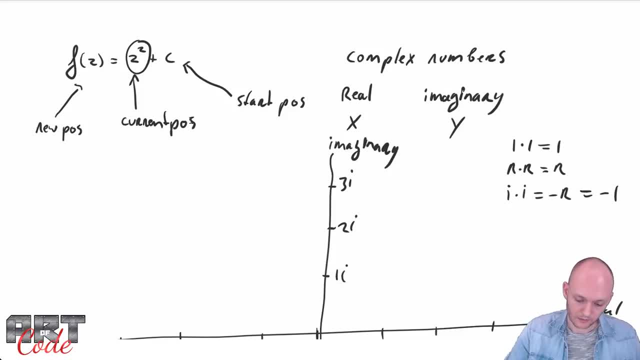 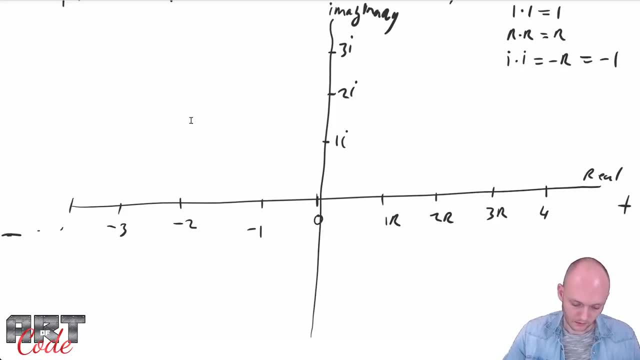 we're taking the, the, we're squaring the number, right. so let's see what happens if we square a number on the real axis, all right. so, um, wait, i can just get rid of the r over here. that was just um to make things more clear. um, so what happens if we square one? well, one squared is one times one, so 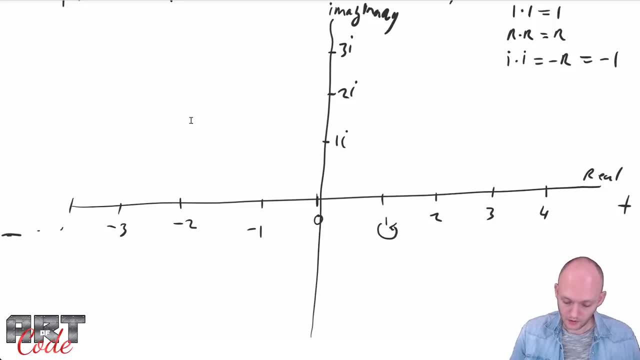 that maps to itself, right. if we square two, that maps to four. right, because two times two equals four. if we would take three, it would map to nine, which is like off to the side over there. okay, great. what happens if we square a negative number? well, minus one. if we do minus one times minus one, that also maps to one and minus two. 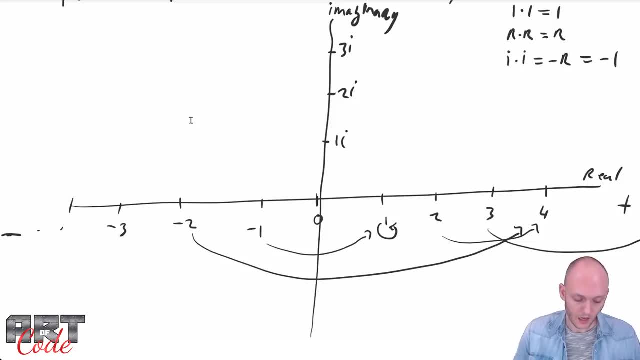 also maps to four. all right, so so it it turns out that any negative number, if you square it, it it kind of folds over the the negative part of the number line onto the positive. so that's a property of real, of real numbers. now let's see what happens if we square an imaginary number. 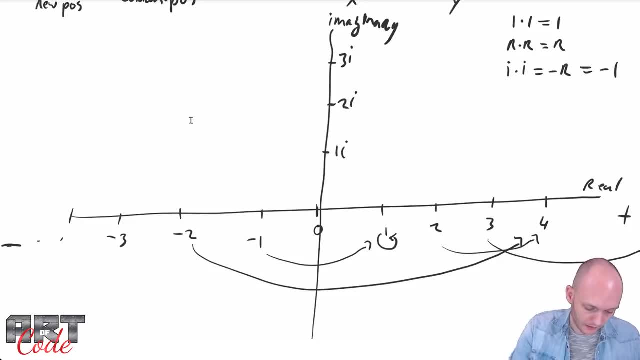 okay, so over here we square one i right, or oftentimes, if it's one i, to just say um, we just say i by itself. well, what happens if we square i? well, over here it says: i times i equals minus r or or minus one right, so, um, so i squared maps to minus one. okay, what happens if we? 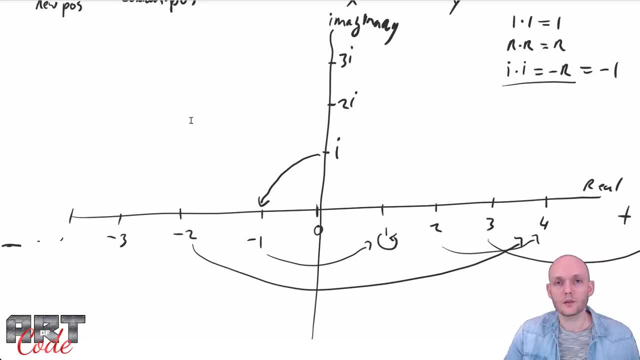 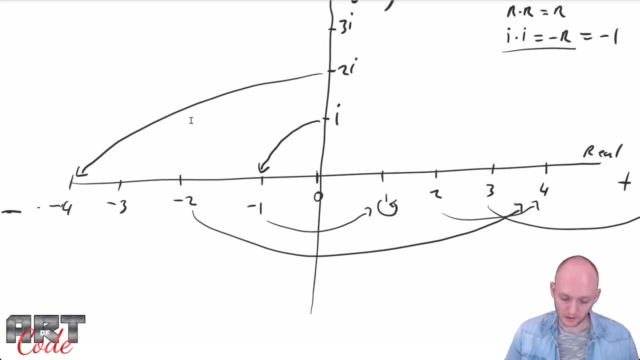 square two. i well, two i is two times two equals four times i times i, which is minus one. so we get minus one times four is minus four over here, right? so two i maps to minus four on the real line. all right, what happens if we have a number, that is, that has a real component and an imaginary component? 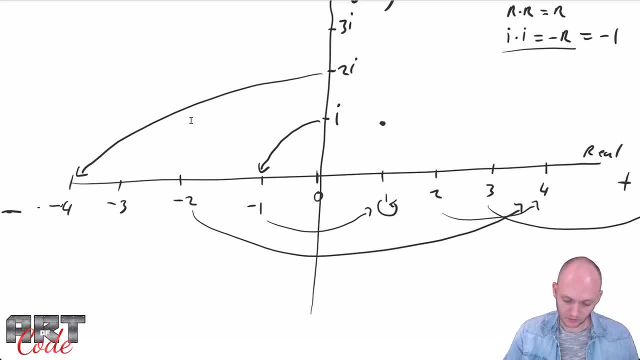 which is a complex number. so let's say this number over here, which would be one r plus one i. right, generally they don't say r, that's my invention. so, and also, if it's one i, then you could just do i by itself, so it's one plus i. what happens if we square that? well, let's see, so we. 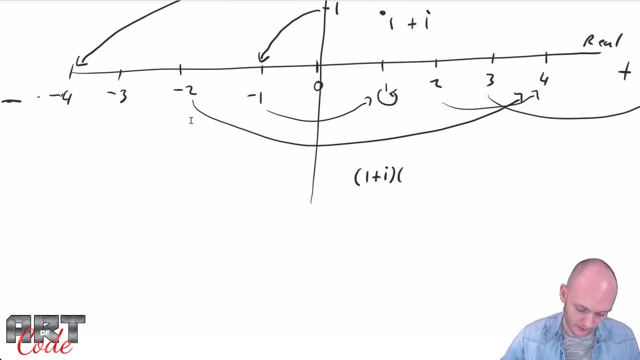 have one plus i times one plus i all. right now we're going to multiply these guys. so one times one equals one, then we're going to multiply these guys. one times i equals i, then we're going to multiply these guys. that's again one times i. 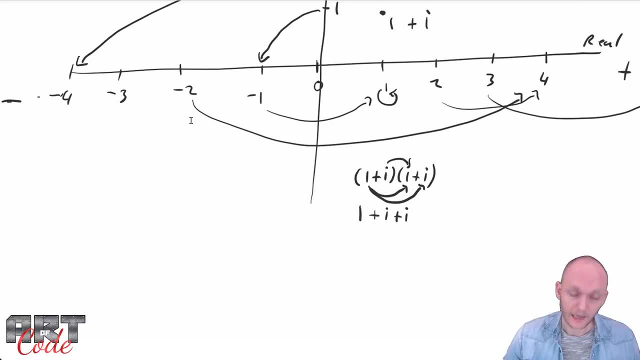 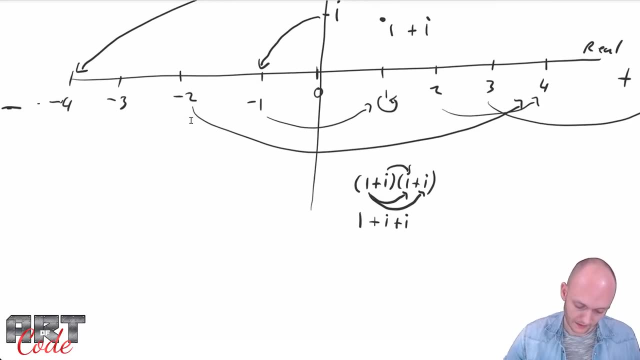 which is i, and then we're going to multiply i times i, and for i times i we have a special rule, which is that it's minus one, right, so i do minus one, and now i have to group them together, so we have the real parts and the imaginary parts together, so this one cancels out with the. 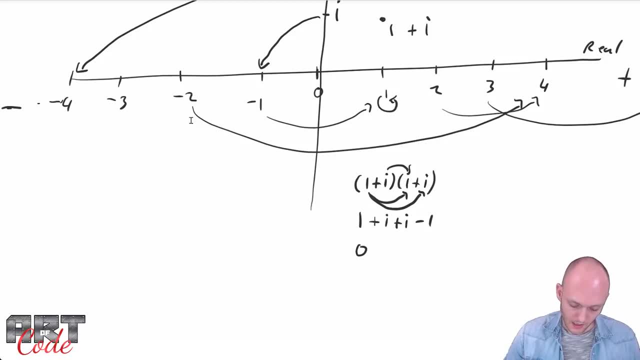 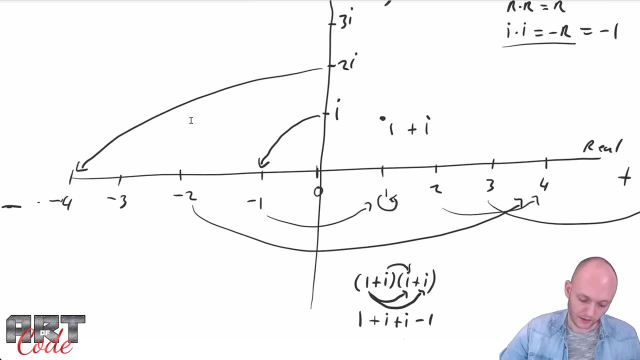 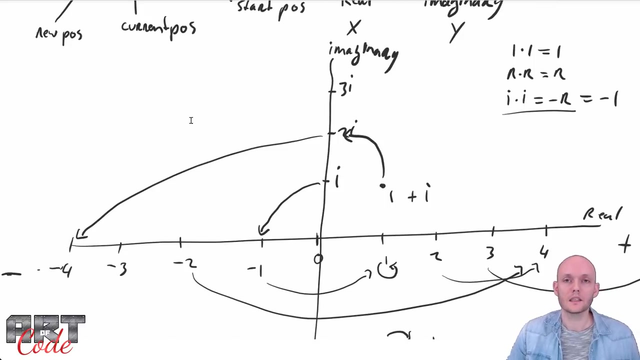 this one. so one minus one equals zero. and then we have plus two times. i okay, so it turns out at this point: one plus i maps to two. i okay, so it looks like, um, multiplying a number by itself, uh, in the on the imaginary axis, uh, gives us some sort of rotation, right? it, it rotates and it scales as. 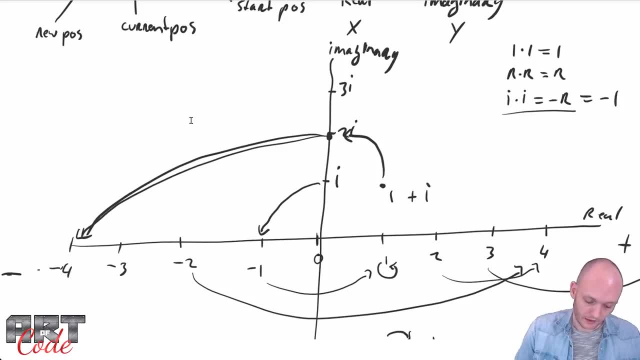 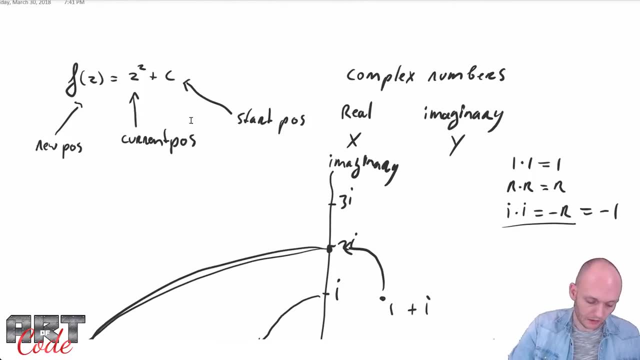 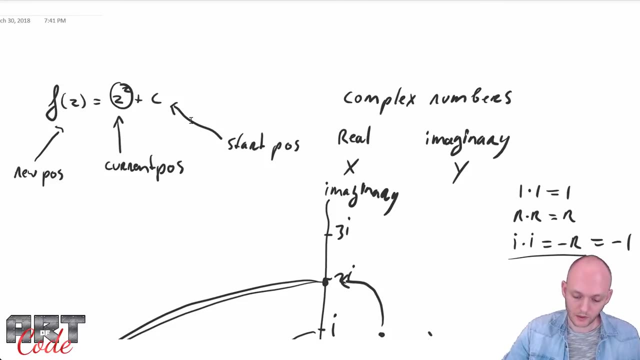 because from from over here to over here it seems to rotate 90 degrees, but it also scales so. so that takes care of of this part. i did it screwed up. that that takes part of the squaring. but we're not just squaring, we're also adding this c value each time. so what? 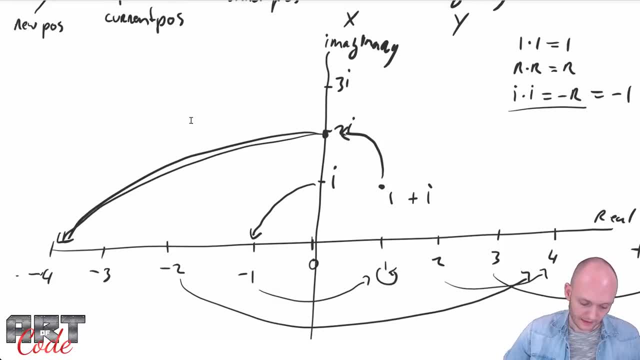 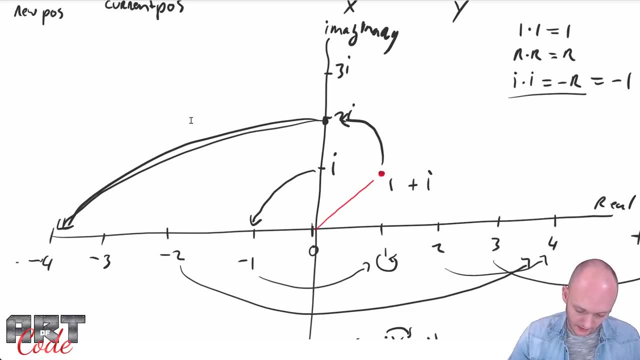 happens to our dancers is that we we start at z equals zero, and then we add our c. so let's say this is our starting position. so our c is like this vector over here, and then at the first step we square this number. so if we square this- well, we already figured out like we get over here and 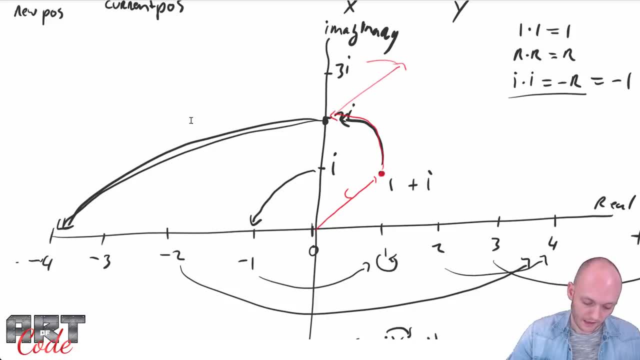 then we add the c again, and then we square that again and we go like we go, let's say, over here, and then we add the c again, and then we like, multiply it again, and then, like we like, we keep going like that, each time we add the original offset and so we get this chaotic dance. 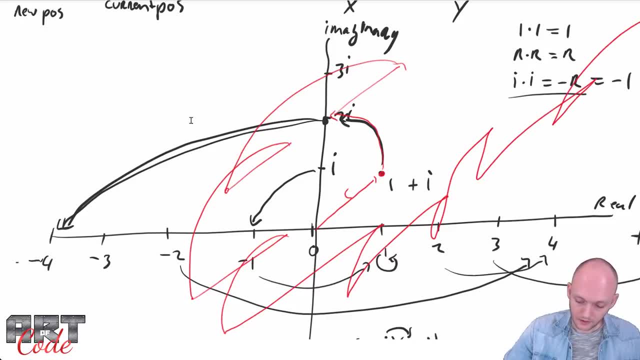 that either it eventually it goes off to infinity over there, or it will stay. it will stay bounded, so, or it will, like, just go inside of here forever, um, but in case of our dancing competition, it will go until the maximum number of steps. so that's kind of how this algorithm works. 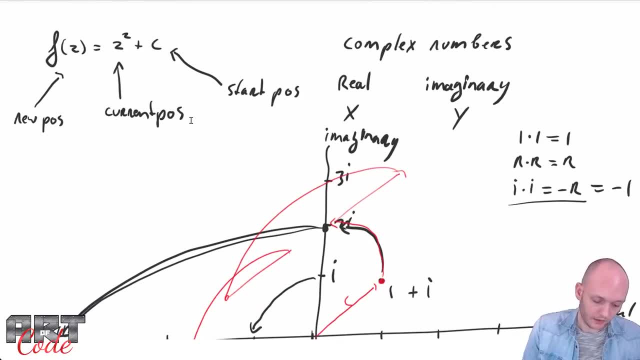 and so now the last thing to do is to figure out, uh, how can we do this complex number thing inside of the computer, which doesn't natively support, uh, complex math? so so for that, uh, we really only have to look at the c, at the z squared over there, so the z 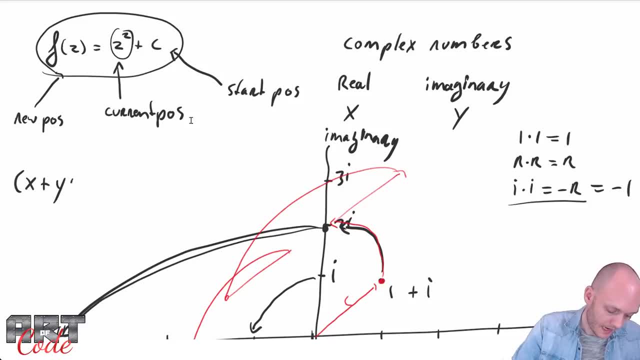 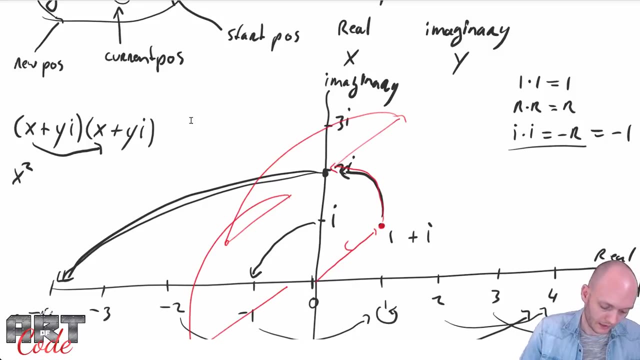 has an x component, right, and it has a an imaginary y component, right. so, and if i square that, i get x plus y, i. so again, i'm just gonna go over here. i do x times x, uh, so they give me x squared, and then this, and then i'm gonna do this one, x, y, so plus. 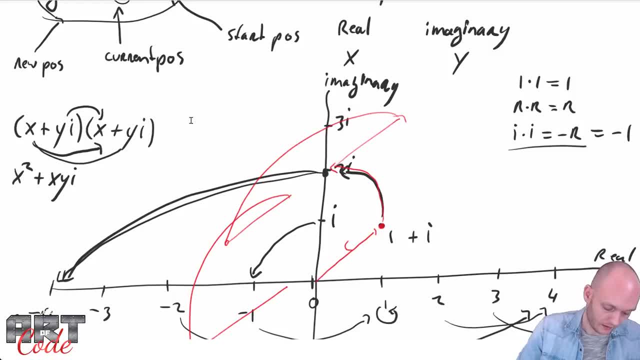 x y i over here. i'm gonna get the same thing, plus- that was my girlfriend- x y i, um. and then- and we have the last one over there, which is y i times y i, which is y squared times minus one. so it's minus y squared right. and now we have to- let me just make some space over here. 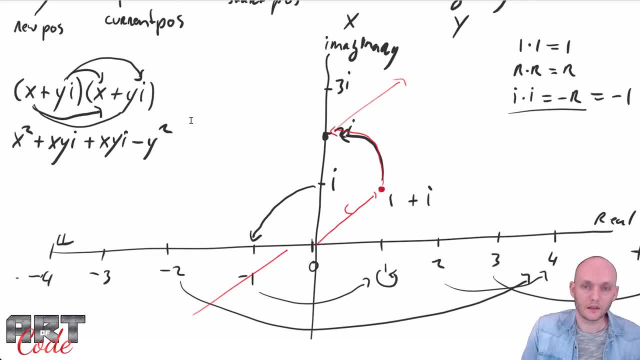 and now we just have to group these together, uh, by real and imaginary parts. so the real part would be x squared minus y squared, and the imaginary part would be 2 x, y, i, if you want. all right, so that is what we can use inside of a computer program. 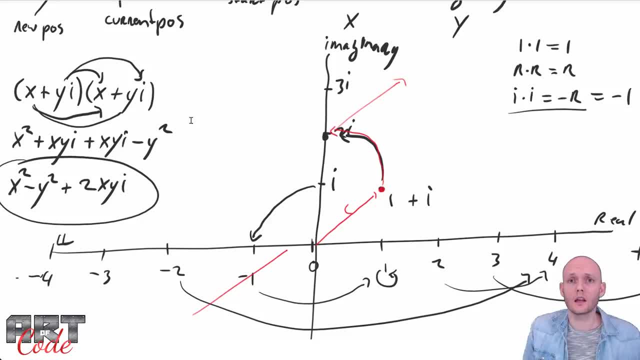 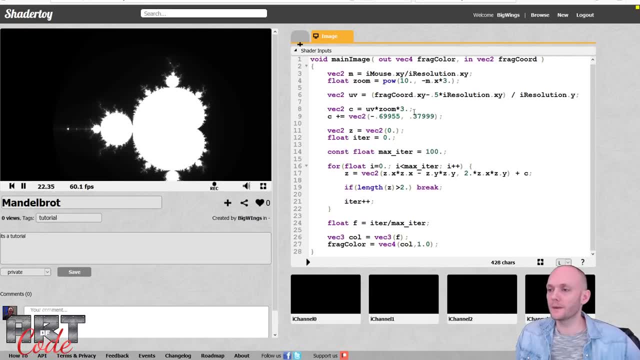 to do this dance step each time. so let's have a look at the computer program. all right, so here we have a manual broad fractal inside of shader toy and let's go through this code over here. so to start with, i have a bunch of code to to be able to zoom this uh, which is not 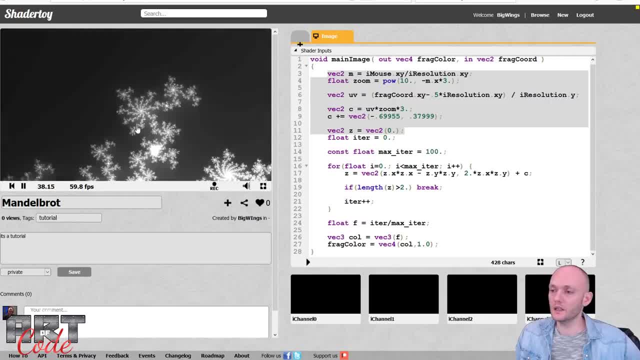 really important right now. it's: it's just uh so that we can see what we're doing, but like the meat of of this algorithm is just over here, so over here we have a a loop that goes uh a number of times. it goes max iter times. in this case it's 100.. this is the maximum number of dance steps. 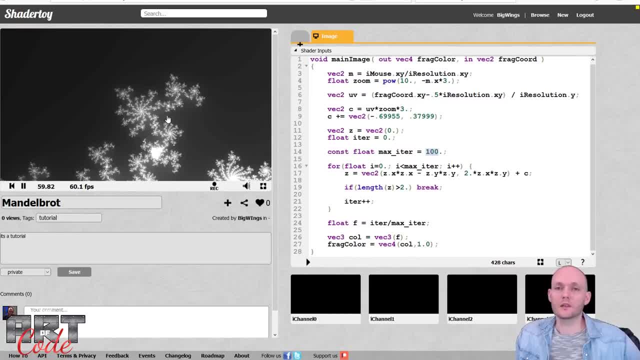 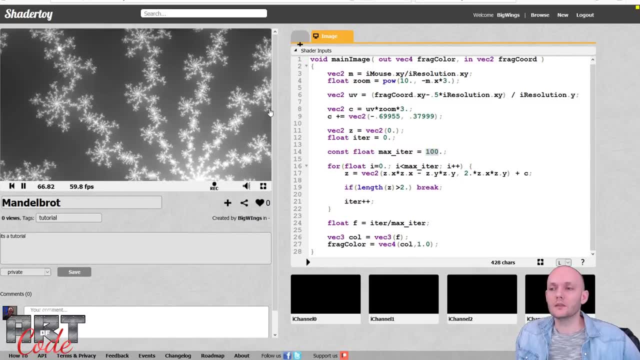 we're going to have so. before we had 20, because otherwise the dance would take too long. but now we can do this higher and the more you want to zoom in- uh, well, here we can't see it. but if we zoomed in enough, then we would need more and more dance steps to get to the other end of the dance steps. 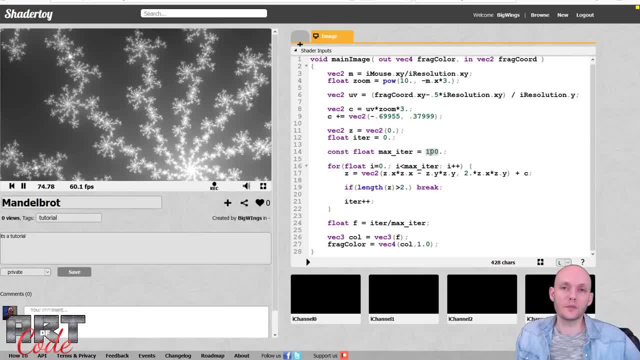 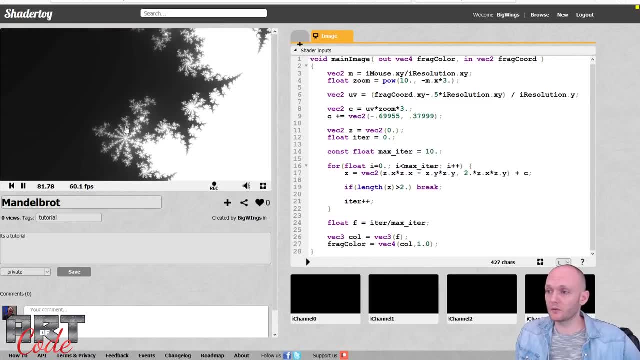 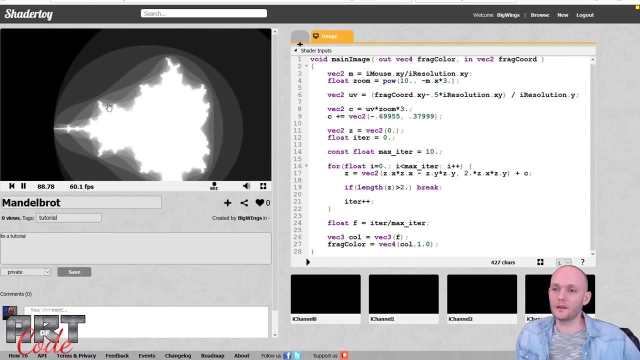 more steps to determine whether we fly, fly off to infinity or we stay bounded, as they say. so like one thing to play with would be just the maximum number of steps. so if i, if i set the maximum number of steps to 10 instead of 100, then you can see that the the like, the 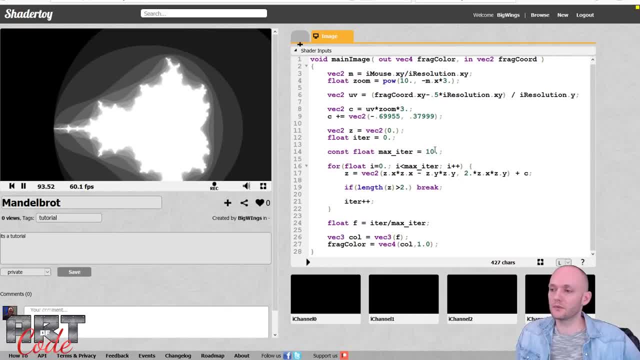 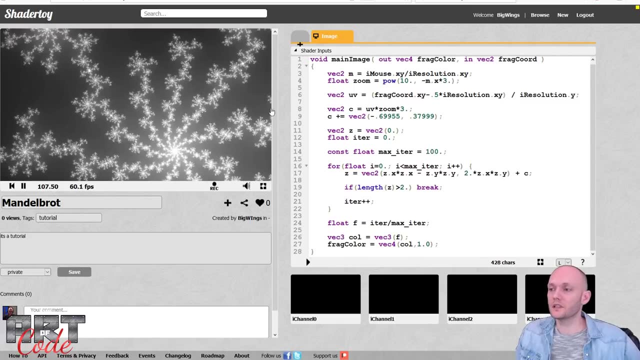 image becomes less rough at the edges, becomes less refined. so let's see what the difference between 10 and 20. you can see it gets. it gets more refined, it gets closer to the actual edge of the of the set. and in order to really get to the edge of the set, you would have to do: 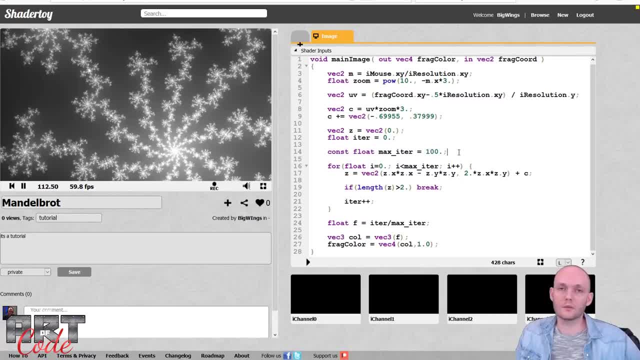 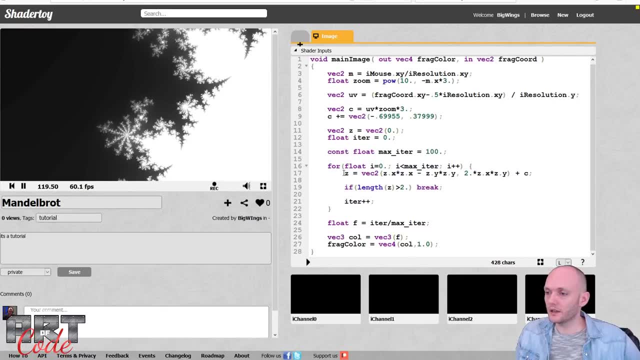 an infinite number of iterations here, which obviously in a computer we can't do, um. so now we're inside of this loop over here and here we have this uh like this: this line of code is is just what i explained, what i explained before. so we we start out with something like uh z equals z squared, uh plus c. 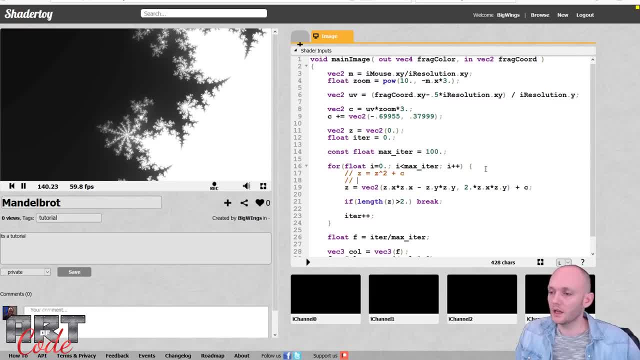 and then we do everything that i explained before, and then we get to this, which this is x squared minus y squared by the x component and y component, and this is, and this is- the new real component of my complex number. and then over here we have two times x, times y. 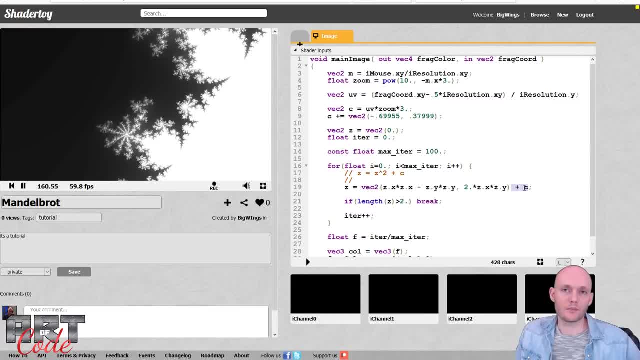 okay, and then, uh, in the end we add the start position and adding. uh, we don't have to do anything special with that because, uh, for imaginary numbers the adding works the same as for real numbers. uh, and then, once we've done that we like, we check. 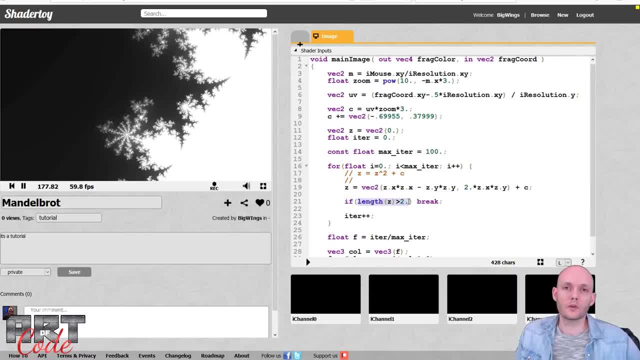 and in this case, uh, it's a little bit different from what i showed before, the dance floor example. here we just check what is the distance, uh, or well, or the length, what is the length of the vector, of the, of the current position, which is basically the distance to the origin? 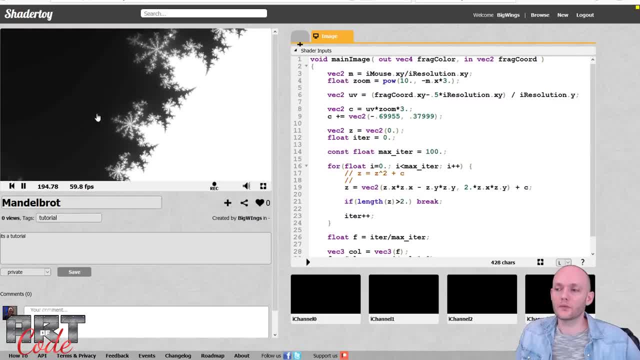 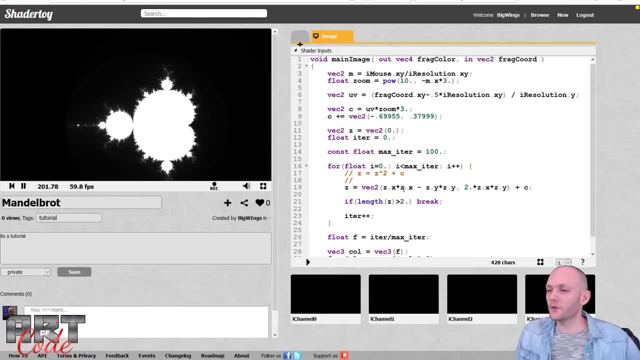 and so this says: okay, if you get farther away from the origin and the origin- i'm not sure exactly where it is on the mtl, maybe over here- if you get farther away from the origin than two, then we consider that you're, that you have escaped. 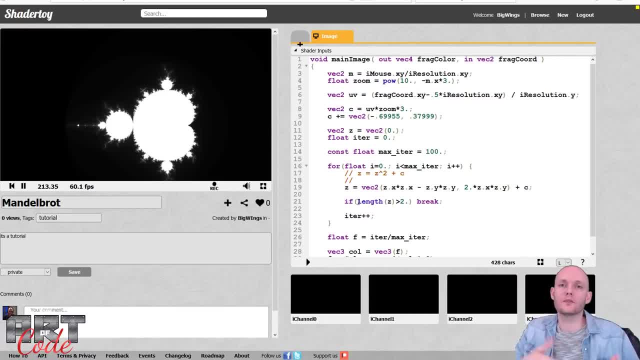 so in the case of the dance floor, like we had a square dance floor, um, so you can, you can play with this as well, so you can change the shape of the dance floor. so in this case, the shape of the dance floor would basically be a a big circle. um, you could change this as well and see what it does. 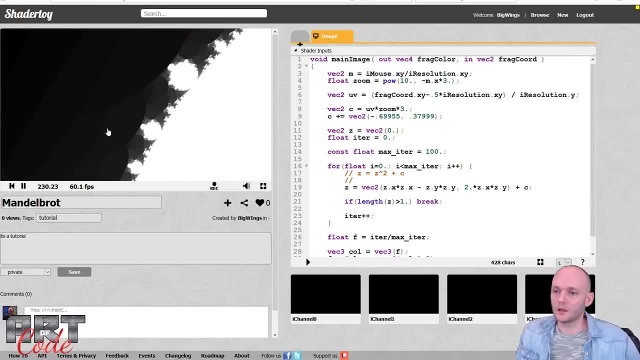 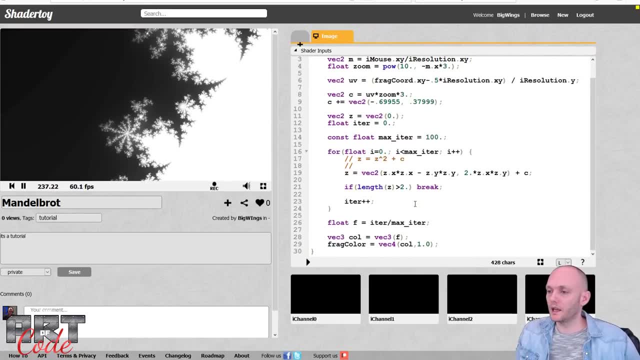 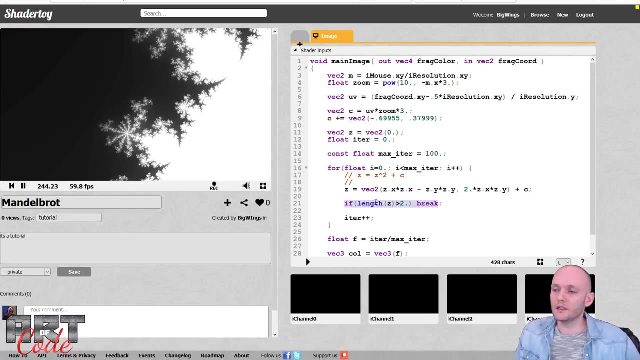 right, so i made it smaller. now and now you have um. you know you have a different looking image, so you can play with the shape, um and um and then uh, each time like it's not, it's still on the dance floor right. each time it didn't get here, um it, it will increase the the score, basically. 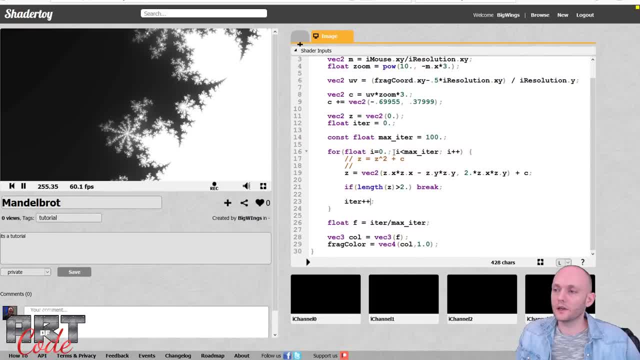 and then, once it gets out of this loop, either by going to the max iteration or by failing this test and breaking out of the loop, it gets over here and here it says, okay, give me this value, f, that is my, my number of steps divided by the total number of steps possible. 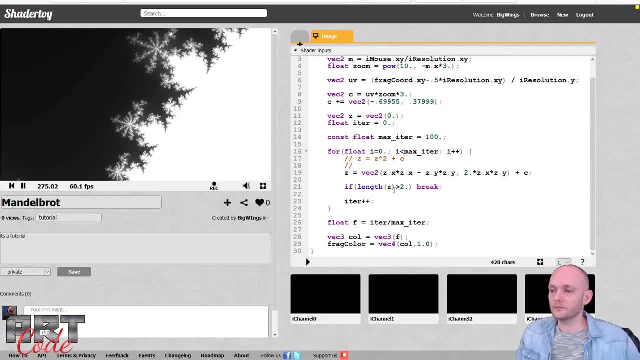 and that is my final, my final color, um, so that's basically how, how the mandelbrot algorithm works, um, but you can screw around with things, right, so, so you could screw around with the dance step over here. so over here i could say: i don't know, let's just see what happens if i, instead of two times i. 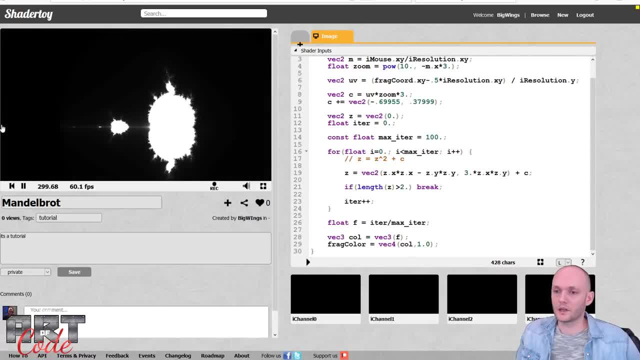 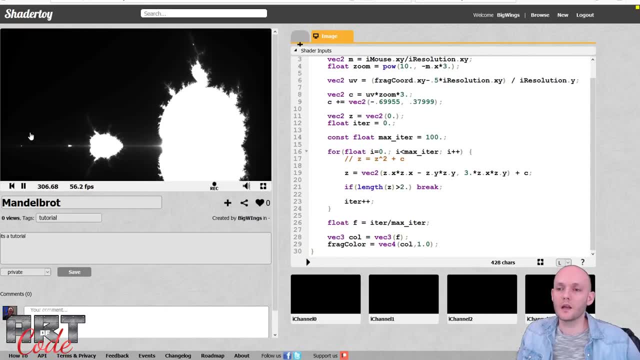 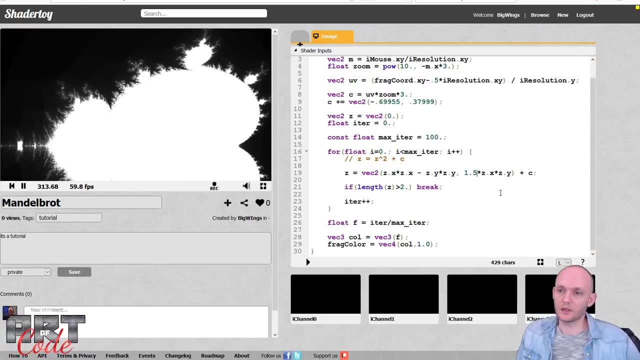 do three times, let's see what happens then. okay, so, where you see, that makes a different mandelbrot set, for which i can't zoom in to a nice uh spot right now, um, but you can play around with that and so okay, so 1.5 maybe, what's what's? what does that give me? okay, that give me. 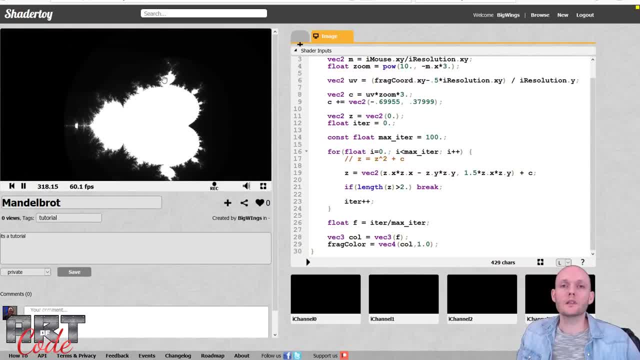 a different shape again. and in case of shaders, because it, because it can do everything in real time, you could even play around with this. so you could even, you could even say: okay, let me, um, let me make a value right here, let me make a value m, let's say, and my value m is going to be an H one. 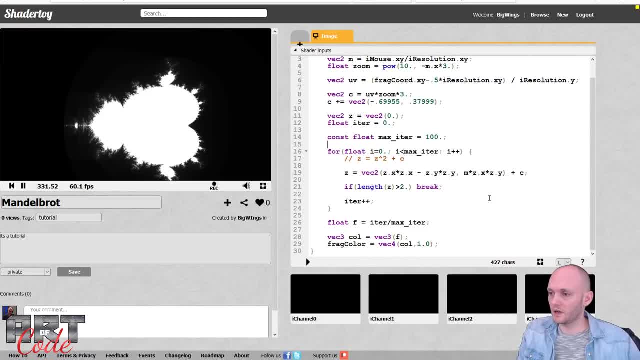 two, three, four, and one, two, three, three, four, four. that's the best view. only one question i did is how do I fit each variables in the & formula and rows and rows and columns and columns. okay, that's all right, just double check. so everything is set in real time, so so. 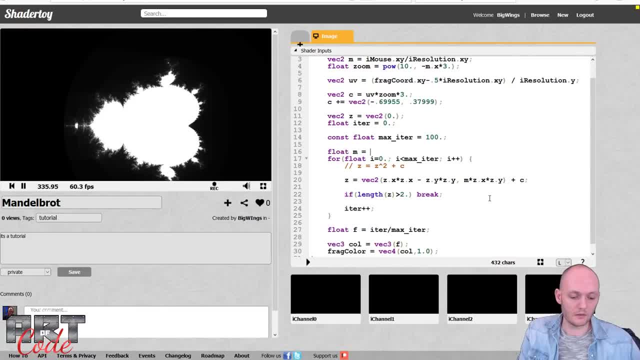 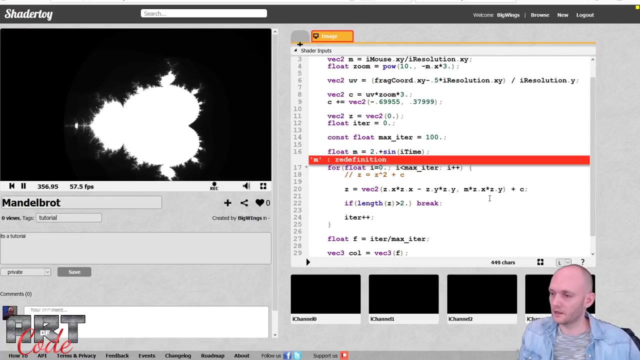 going to change. so i'm going to say: float m equals like mix of. let's say: okay, the original value was two and the new value was uh. well, actually, no, here, let's keep it simple, let's just do. let's just do two plus the sine of i time. let's see what that does. okay, i already used m, so let's. 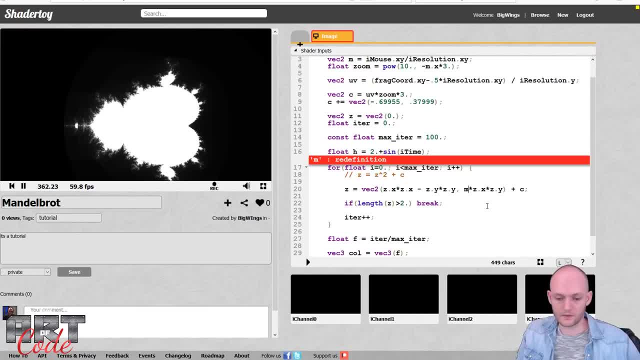 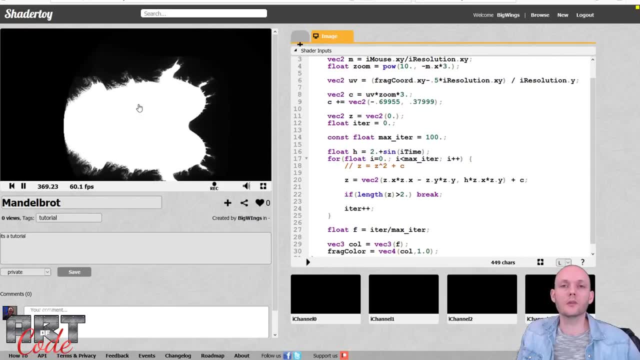 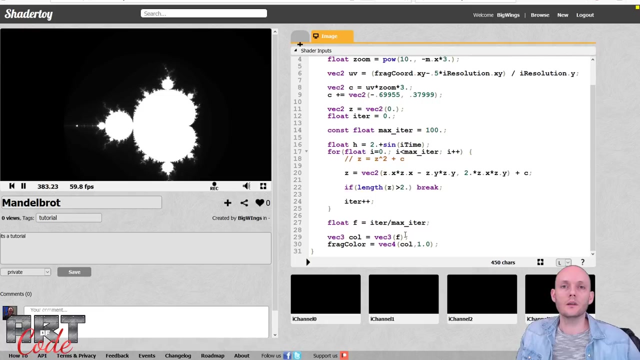 use a different one. let's say h and then over there h. all right, so i can morph things now so you can see this is a. this is a fun thing to play with, um. so that's, that's changing the. the dance step, um. so let me just put this back to where it was. another thing we could do is change the the. 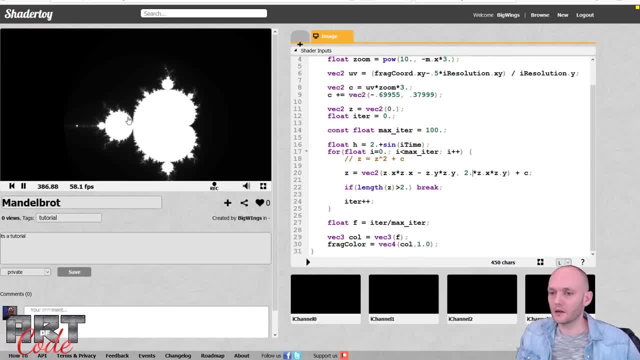 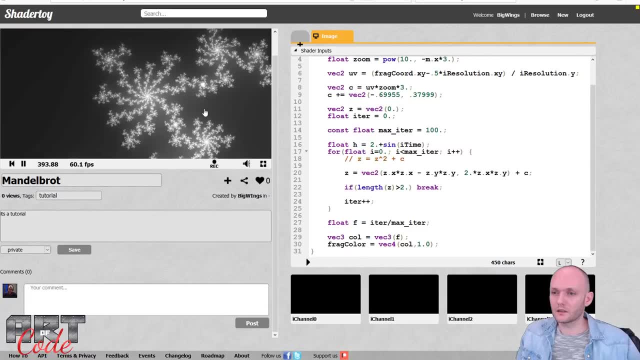 the visualization of the of the color. so right now, uh, it's pretty much white now, so let's change the color. so let's change the color, so let's change the color. so let's in the middle and black pretty quickly when you get outside. um, but it's not, it's not completely. 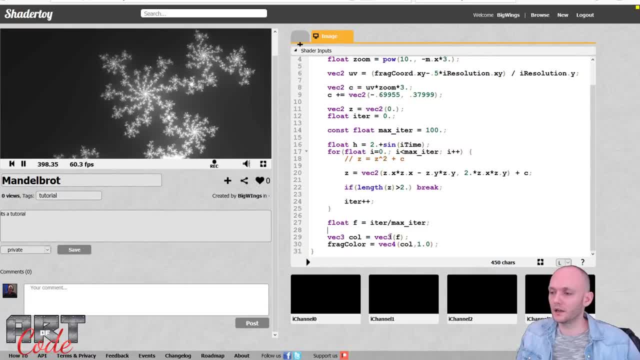 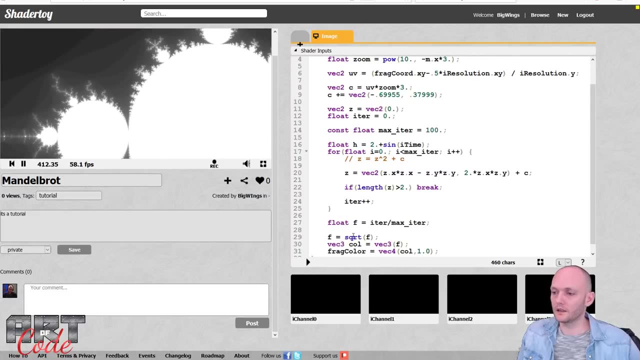 black. you can see that, that there is a gradient, right, well, we can play around with that gradient. so i can say over here, for instance, f equals, let's say, the square root of f, to kind of stretch that gradient out a little bit farther so you can see, you can see more, right, i can, i can even. 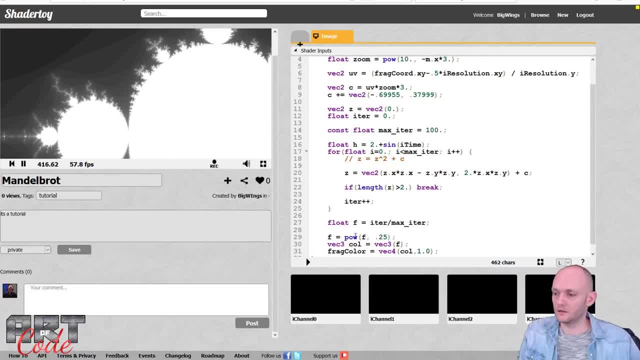 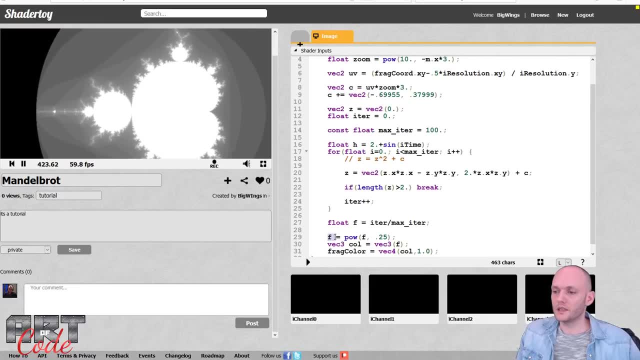 stretch it out farther by uh like doing something like this. all right, another thing that i could do is i could use this f, because this f value goes between zero, zero and one. i could use this f to look up a color from a texture. so let's try that real quick. i don't. 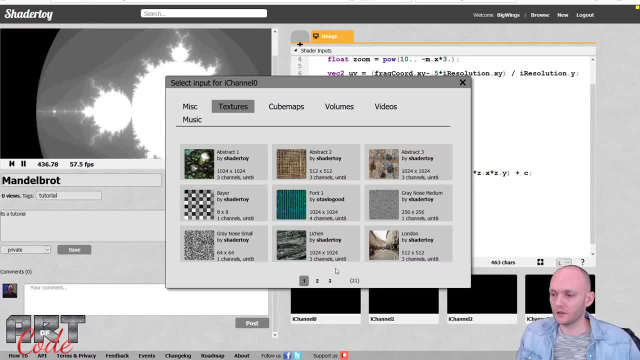 really have that many exciting textures over here, uh, but if you can make your own texture, then you could make a bunch of textures and you go to photoshop and you add a bunch of gradients and now you can have- you can select- many different gradients that you can use. 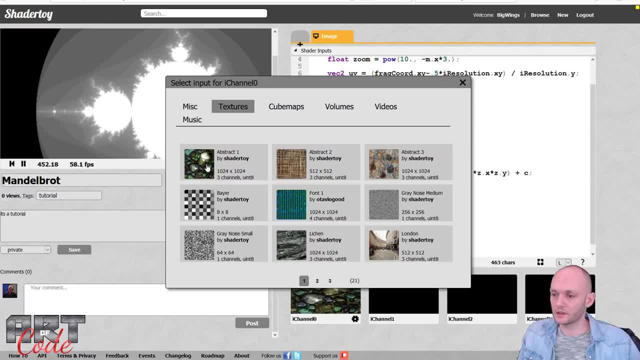 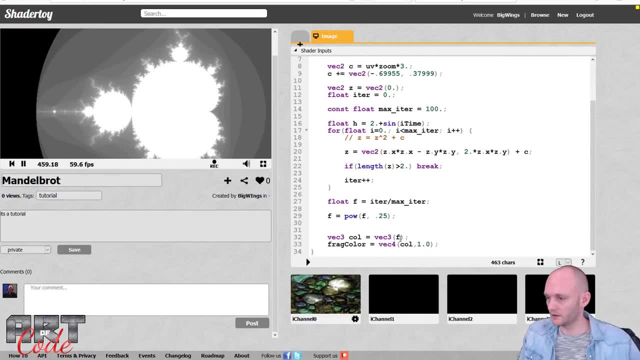 but for now let's just say, okay, i take this one over here, this, this texture, and now i can say: so, let's say over here, i do no, hang on over here, i do texture. i hope i do that correct, because i never use textures. i channel zero and then i have to make some uv coordinate. so let's. 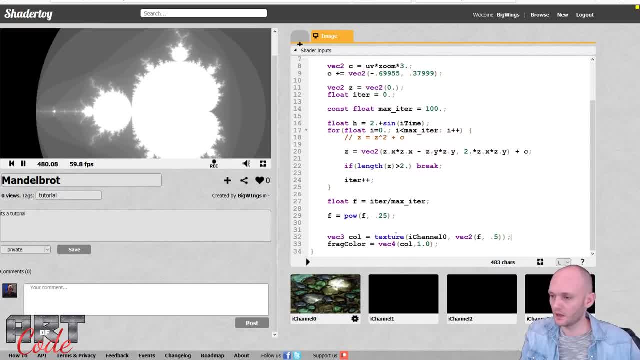 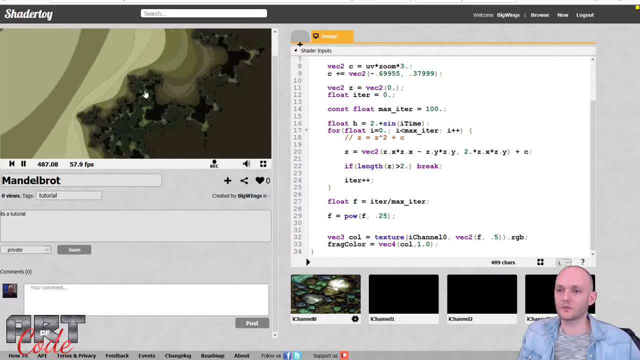 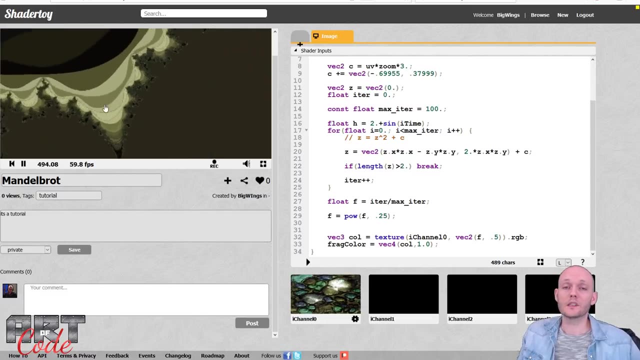 let's use f for the uv coordinate and then rgb. so let's see, okay. so you see, that creates some sort of weirdly colored situation and you can play. you can play around this, around with this and get lots and lots and lots of different types of effects. um, let me put it back to where it was, so i'm just gonna go back. 3f. 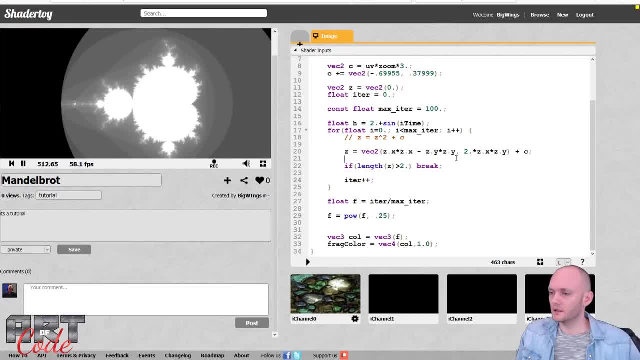 um, let me see here one last thing. perhaps, uh, we could, for instance, uh like, instead of checking, uh, instead of just checking whether we're outside of the dance floor, like we could have one judge, uh, check, um, how, what? what was the closest that we got to the x-axis or to the y-axis? 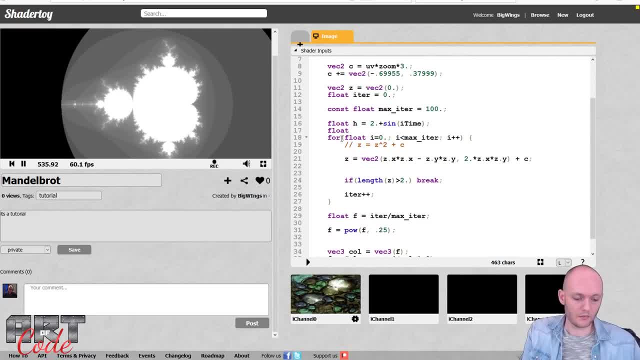 so, so for that you could. you could do something like: uh, you, you make, you make a, you make a value over here, you set it to something large. and then over here, uh, you say, okay, ma equals the min of ma and the absolute value of, let's say, the x component. 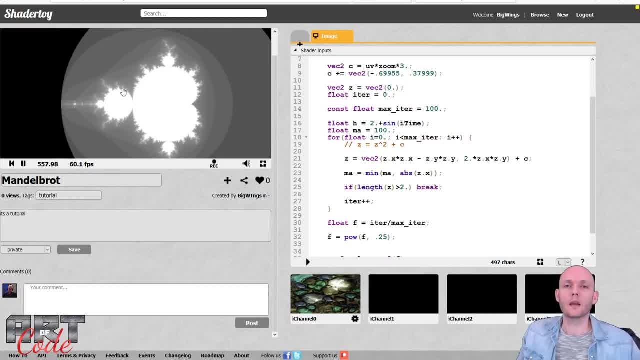 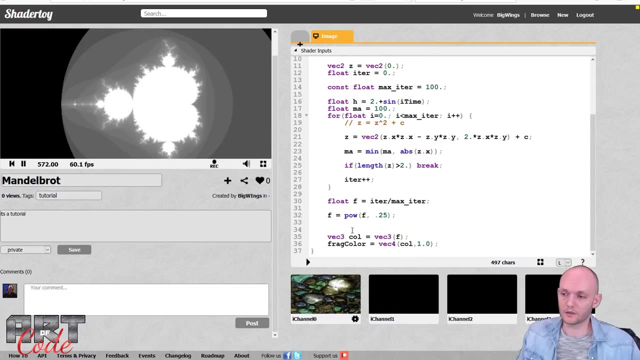 um, so this keeps track of which dance step came, came the closest to a certain location, or in this case, to the um, to the um, uh, to the horizontal axis in the middle here and then um, And when we get out of here, we could use that to do something. 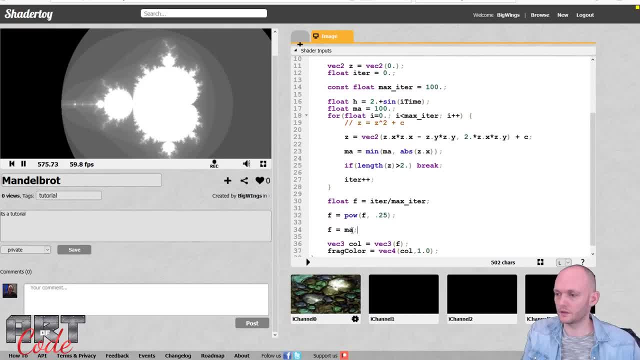 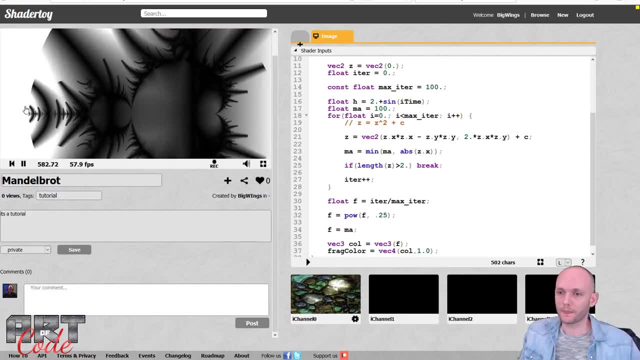 So let's see here: f equals ma, and this is off the top of my head, so it will probably explode. Okay, well, there you go. So here we have different kinds of patterns now and we can combine those and we can. 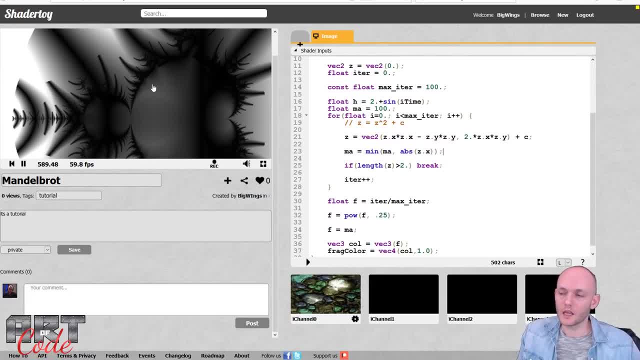 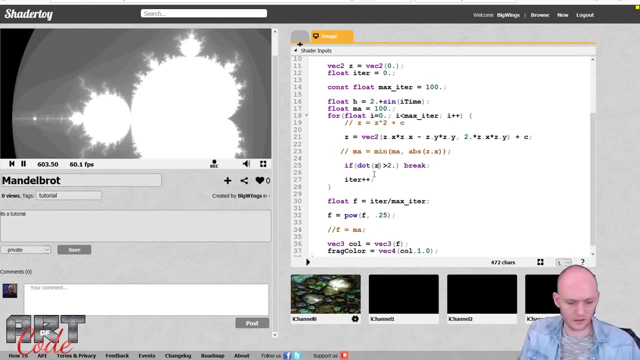 come up with any kind of rule, basically to come up with different images, And you can really get lost in this and play with this for a long time. There was one yesterday I was playing around with where I did this: I think c times c.